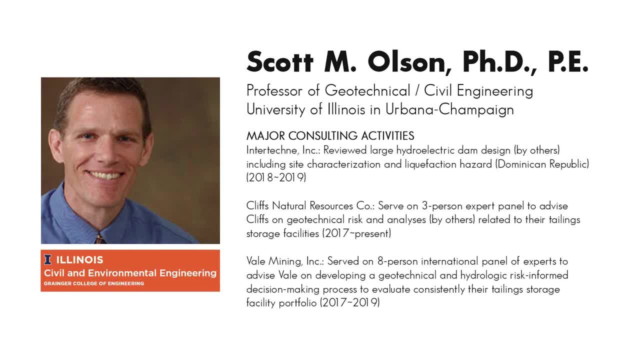 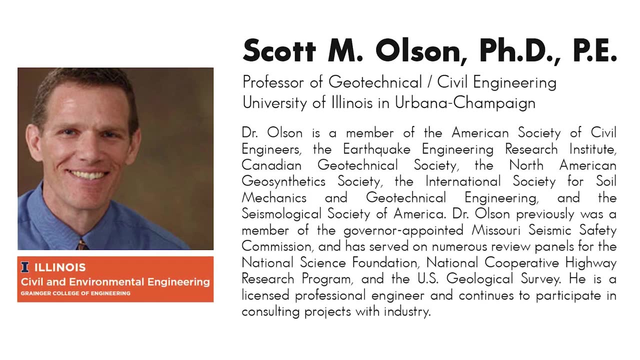 foundation structure interaction. From these activities, Scott has published over 140 papers, journal papers, conference articles and reports and has received numerous awards for his research and teaching, including the ASCE Arthur Casagrande Professional Development Award and the Walter L. 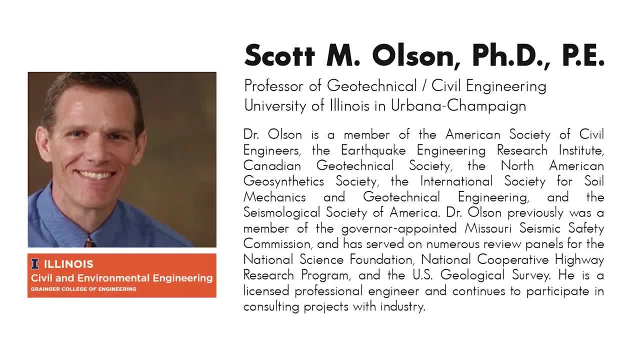 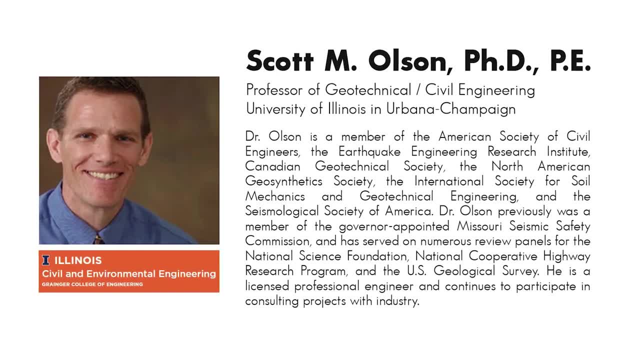 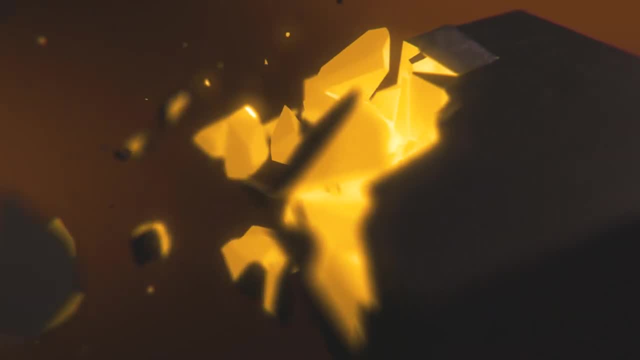 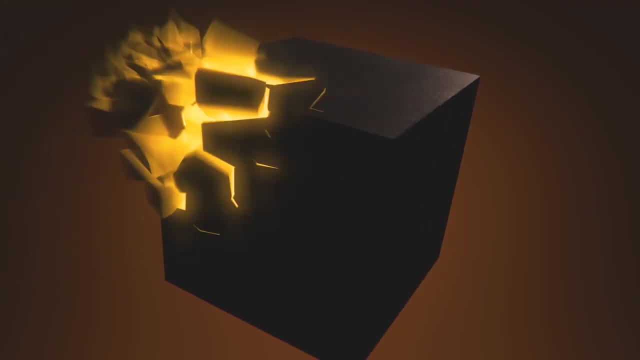 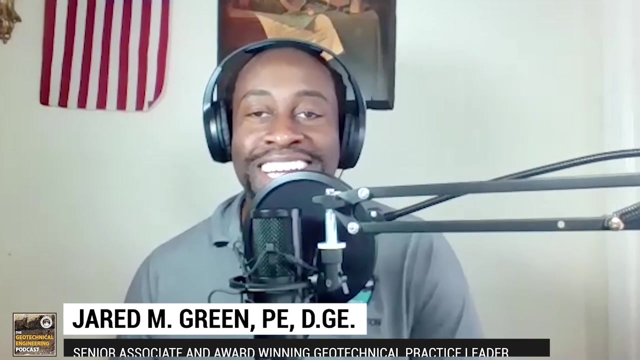 Hubert Civil Engineering Research Prize and the Canadian Geotechnical Society RM Quigley Award. He is a licensed professional engineer in the state of Missouri And with that let's get right into our conversation with Professor Olson. Professor Olson, welcome to the Geotechnical Engineering Podcast. We are. 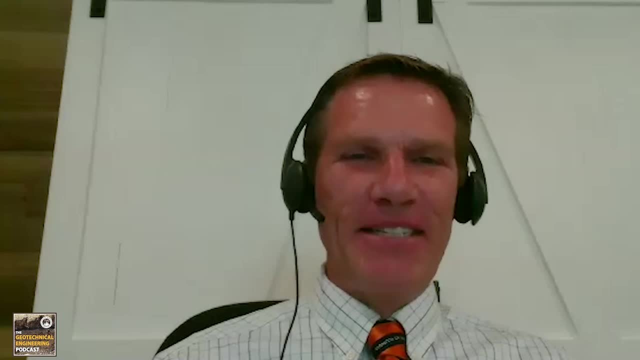 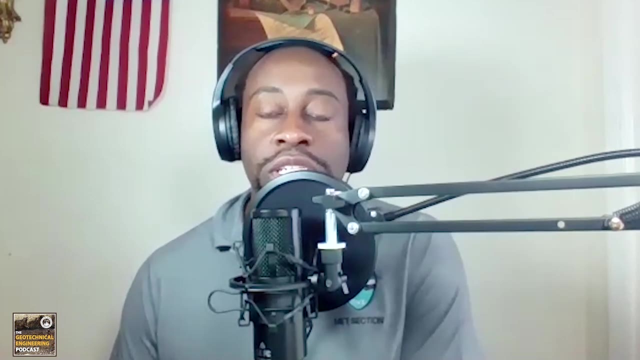 honored to have you. How are you feeling? Doing great, Jared. It's nice to see you again. Excellent, Excellent, All right, Well, if you could, you know we introduced you earlier in the show, but, in your own words, can you tell our listeners a little bit more about? 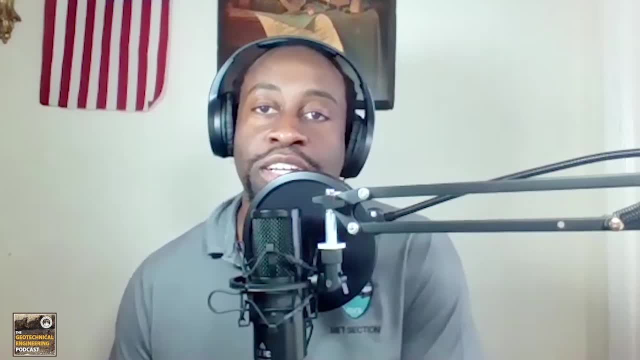 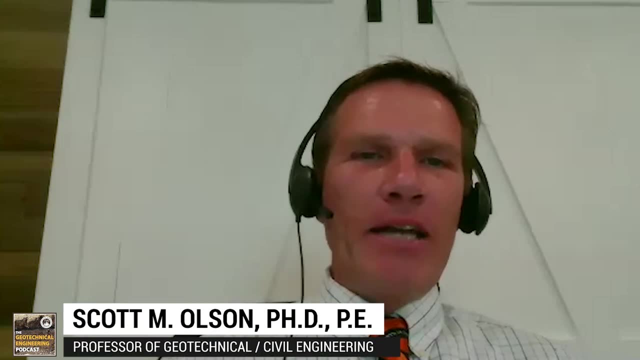 your work. Can you tell us a little bit about yourself and some of the things you do at your job at University of Illinois, Urbana-Champaign Sure? You mentioned that I'm a professor of civil and environmental engineering, but you know, while a lot of students and other professionals have some impression of what they 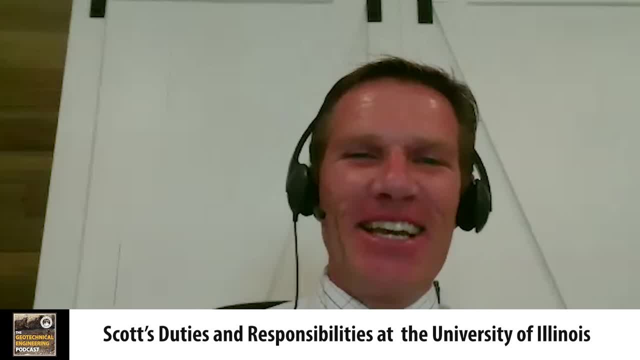 think professors do. I don't know that necessarily it's the right impression. Of course, you know, the first thing about being a professor is education. We want to develop and train the very best next generation of geotechnical engineers and engineers in general. 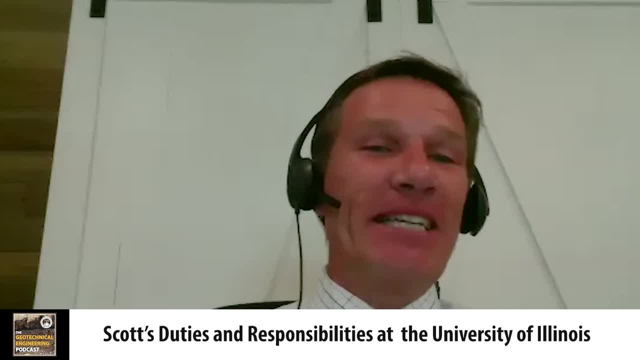 And I think that's a great example of what we're doing. I think that's a great example of what we're doing. I think that's a great example of what we're doing. Hopefully I'm a decent example of what that education can provide to you. 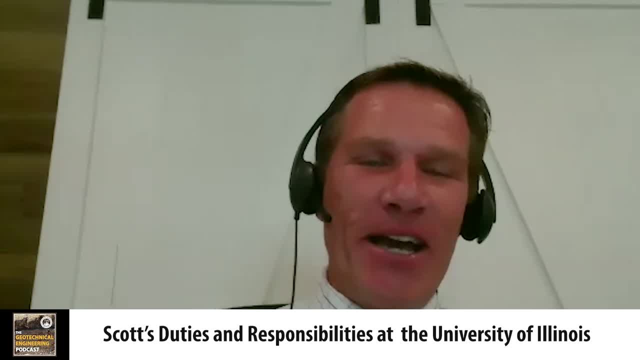 On top of that, we're doing research year round at Illinois. A lot of folks say, well, you just had the. you know, you get a long summer vacation here. You should really be out enjoying yourself. And I'm like- no, I'm just like you. I'm down in my basement right now. 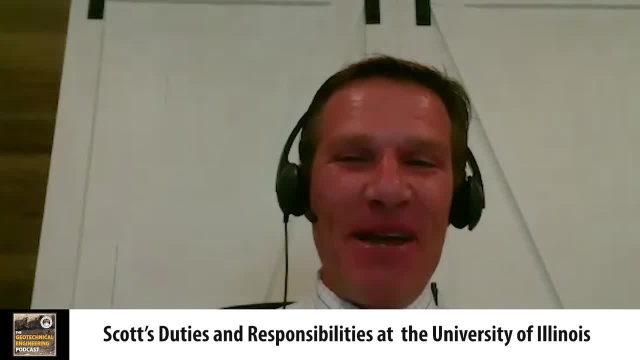 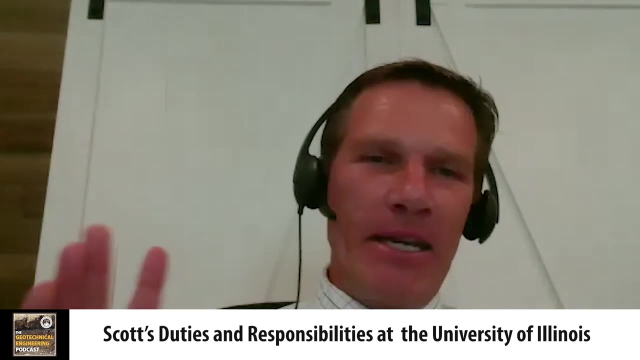 doing research, you know talking with my students and writing papers, And so you know my main focus in terms of research is conducting and publishing research. that's really going to impact practice, at least the niche of practice that I'm engaged in, So I don't really get into the esoteric stuff. 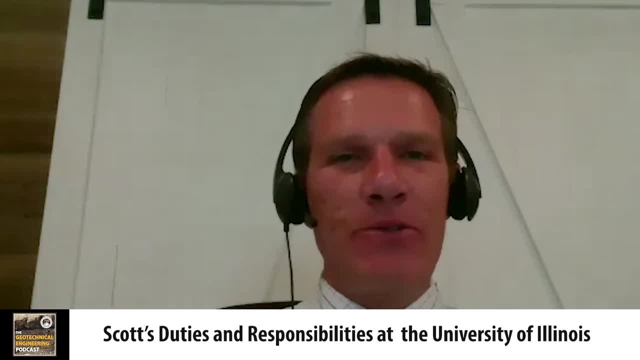 And it's never really been that interesting to me. Fundamentals, certainly. I'm going to mention that many times. I imagine how important that is. But I want to have, or I want to conduct research that's going to impact practice, that's going to change the way we do things as practitioners. But of 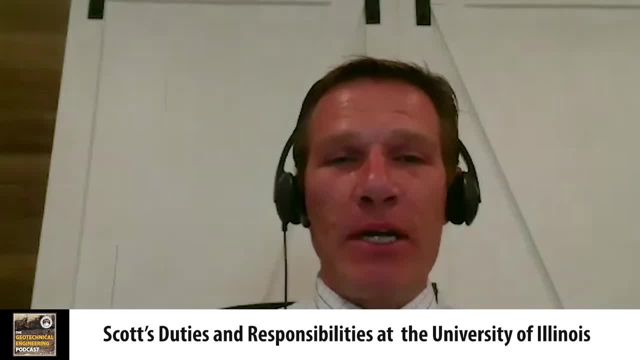 course there's mentoring. You know you think of mentoring as something that when you get out into practice you have a supervisor or someone else that mentors you. But of course we're mentoring students and PhD candidates and postdocs at the university level to helping them develop. 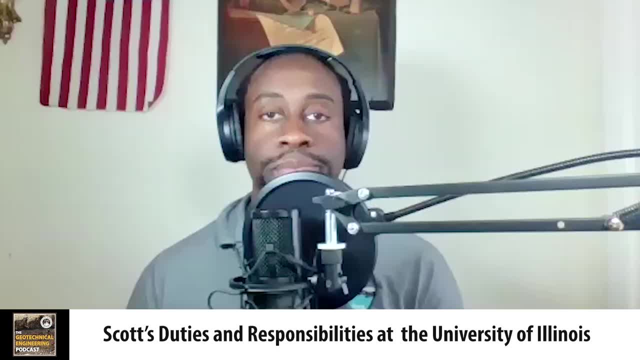 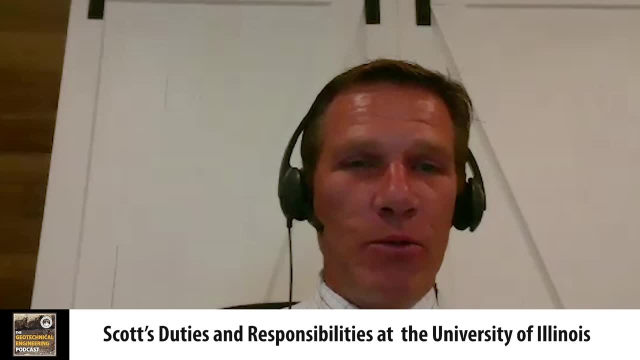 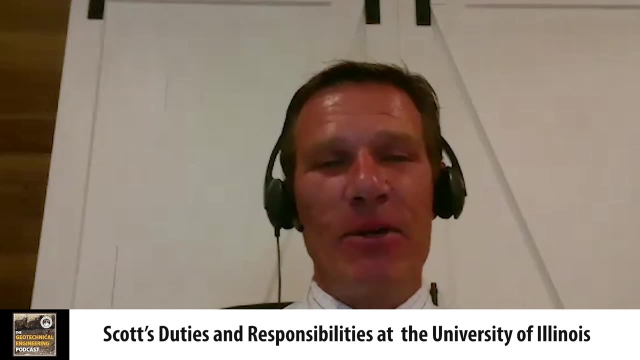 and decide on their next career step, whether that's going into practice or going into academics at some point. Service is a really important piece of what we do. Definitely We have to participate, And for us it's an obligation, more so than- or, hopefully, it's also. 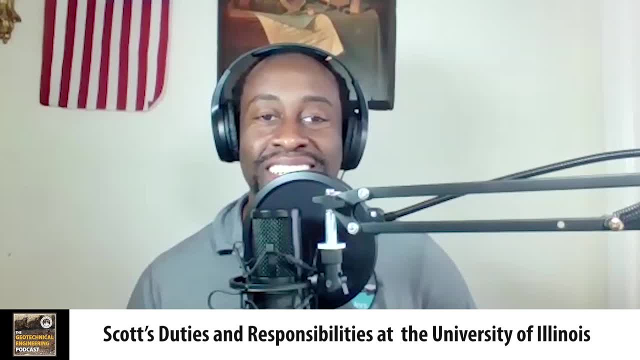 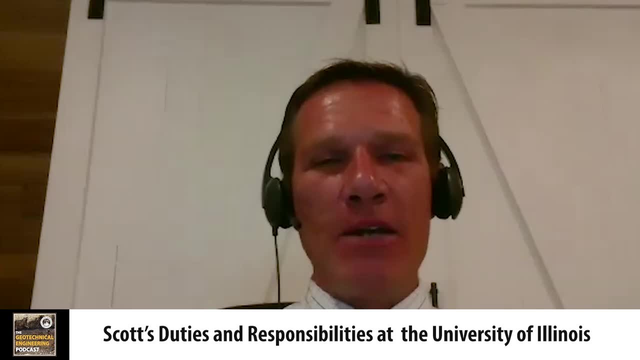 a desire but it is an obligation to some extent, to get involved in those non-university related things, from serving on committees to working with national technical committees, to doing all those things to make sure that we project the right image of our profession and make sure that. 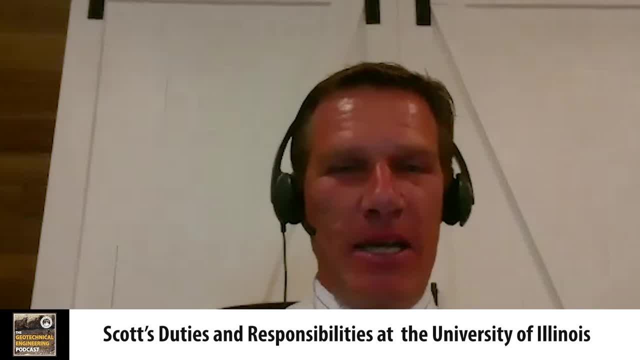 we give back to more than just our students and our students And the university, to kind of broaden our reach. And then, of course, practice is still an important piece for a lot of faculty members, myself included, that I get like to stay involved. 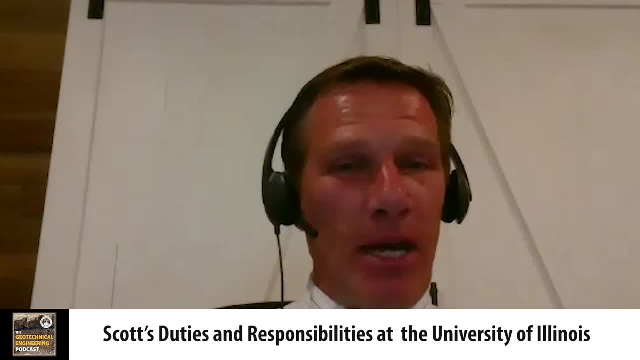 in consulting work and in practice, so that I know what's going on And so that I can offer my students a little bit different perspective on what the next step of their career might be. That's awesome. That's awesome. And when you think about your career, 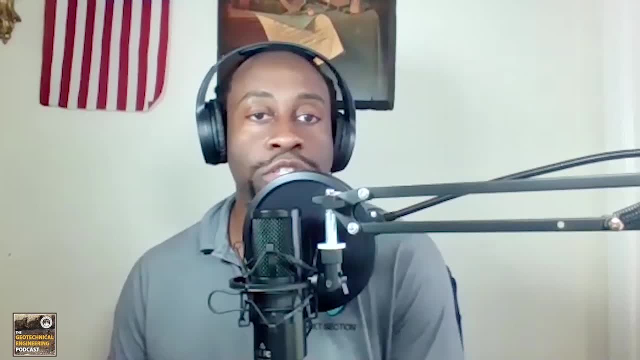 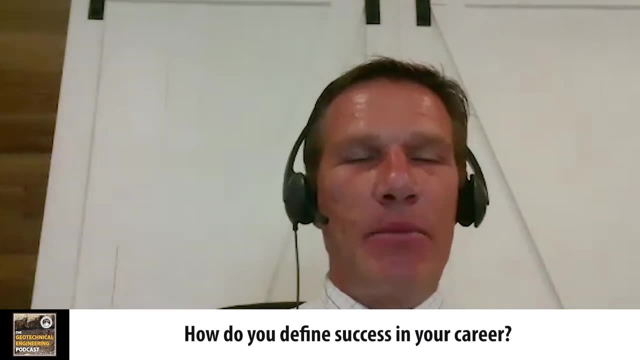 I would say that you've had a successful career. How would you define success In your career from? for me, it's, you know, the first, first and foremost. it's that my students are doing well, and that's both the students that I'm doing research with, but also just the students. 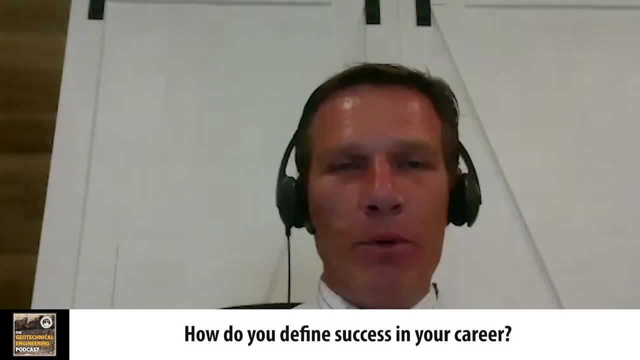 in my classroom that I want to make sure that they are well prepared for that next step, So that if they go out to practice they are ready to work on the most challenging projects that are out there And hopefully then, if I prepare them well and they get involved in these projects, give me a call. 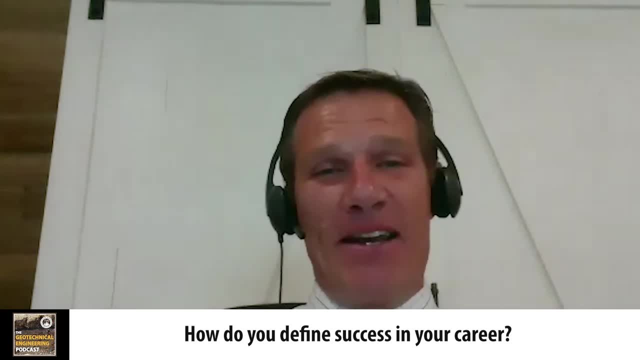 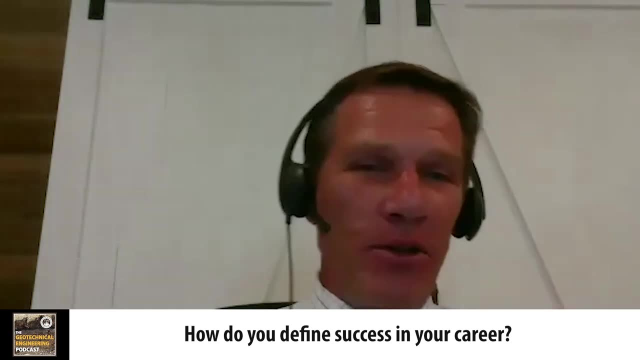 and say: Hey, I'm working on this stuff. Can I give a talk about it at Illinois, Or we need some help. Can you lend us a hand on this particular project? So again, it kind of all is circular so that I can. 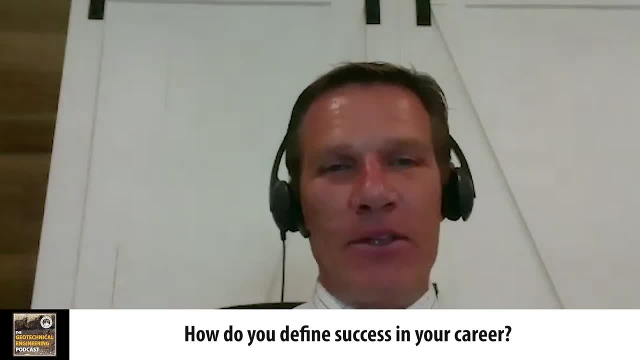 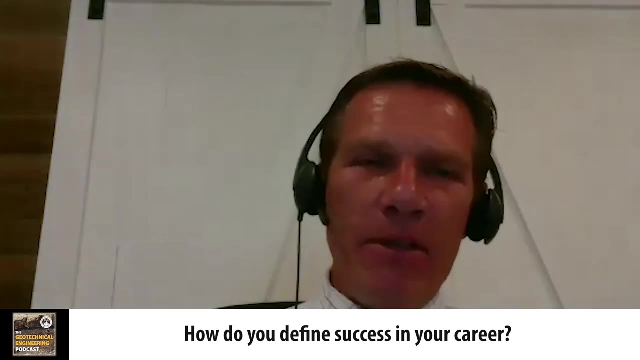 remain active and remain involved, but I want to get those students out there as part of our profession. And then for myself, my metric is that my research again is having an impact on practice. that I see It's not about seeing your name, but it's about having that. 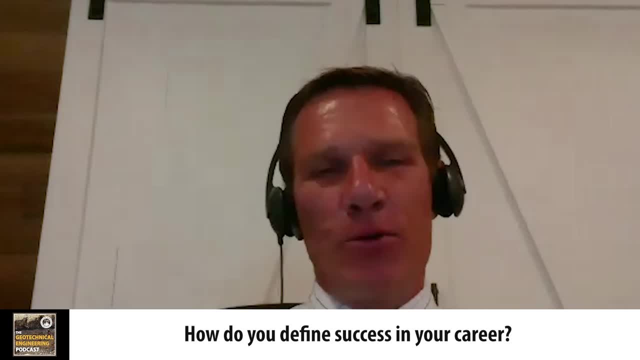 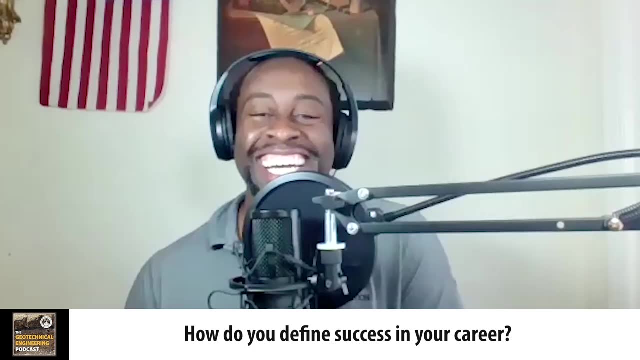 impact and making sure that what you're the time that I spend doing research- and my wife tells me I spend a lot of time doing that sort of stuff- She reminds me how many hours that it's actually has some value and excellent to be utilized and not just stuck on a shelf somewhere in a book. 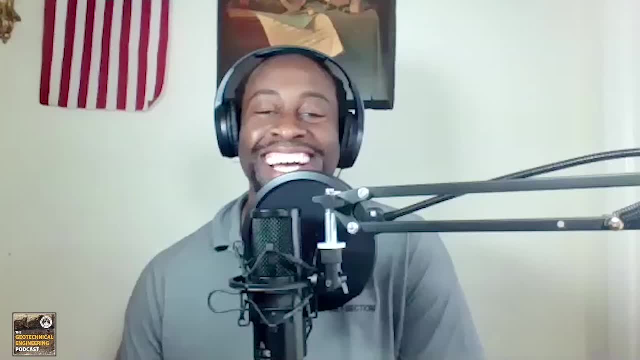 that nobody picks up for the next 40 years. No, we don't want to do that. We don't want to do that. Yeah, I remember when you reached out to me when you were getting ready to put together a Geo-Congress. 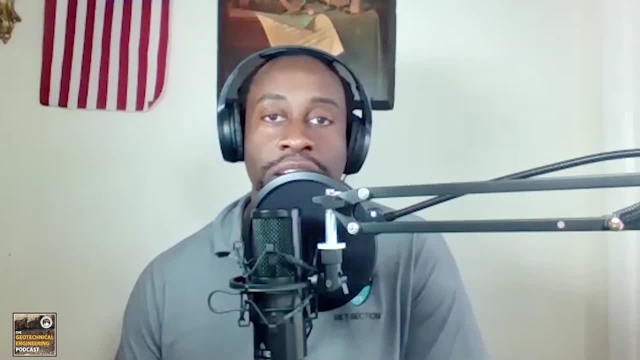 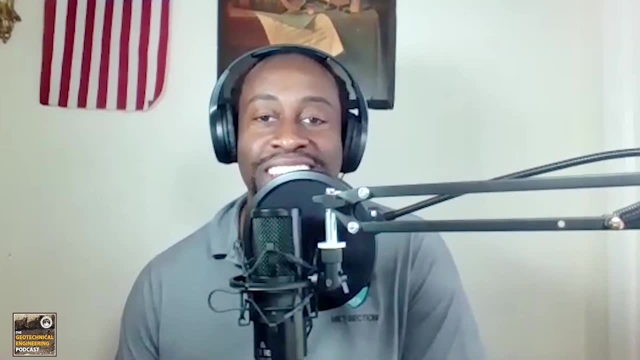 when it was going to be in Philadelphia And although we didn't, we kind of just missed each other at Illinois- when I was graduating is when you were starting, but it was awesome to work with you putting that together And it's so much that happens behind the scenes And it's fascinating. 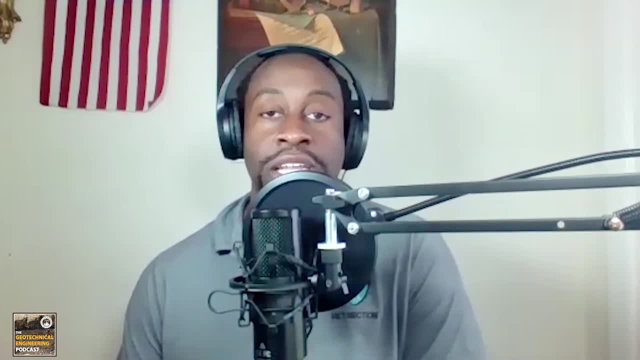 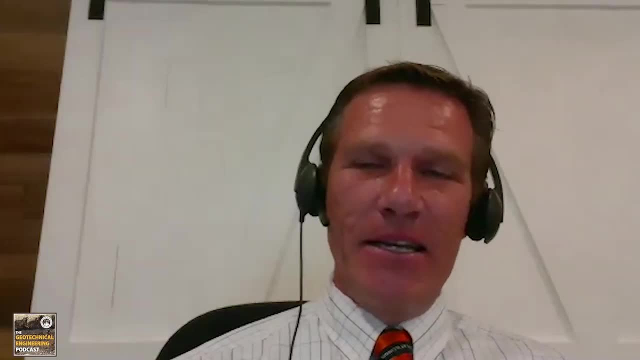 that even as a professor, you're tasked to do these kinds of things, and it forces you to tie back to industry, which I think is good for both sides. Exactly That's the intent. I don't really know, being a three-time graduate of Illinois myself. I 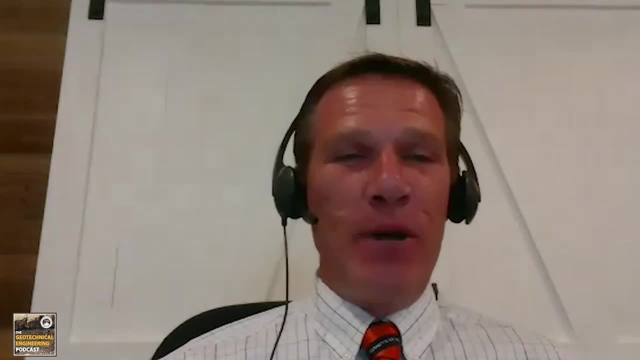 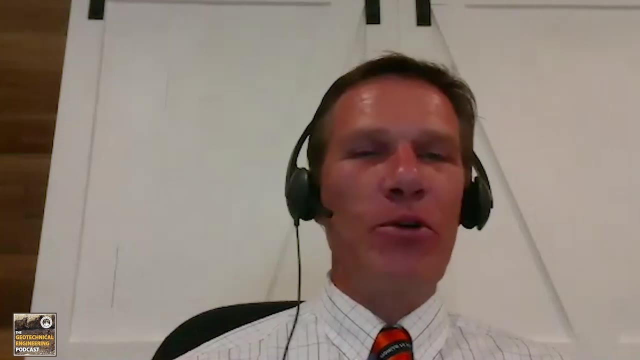 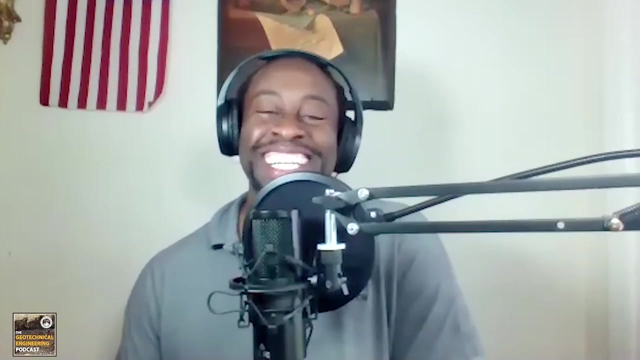 don't really know what other programs, why other programs, would do anything differently than have that handshake between industry and academics be as strong as possible. You know we don't get to shake hands as often as I'd like to anymore, but definitely that handshake should always be. 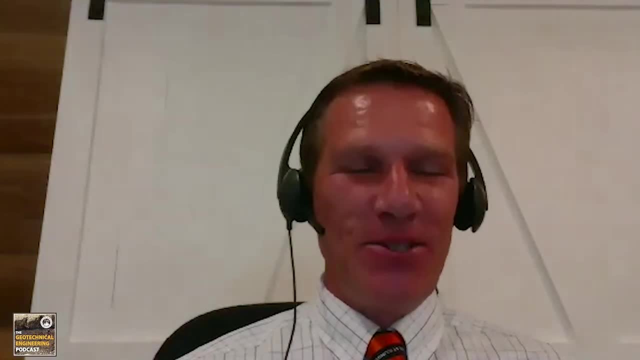 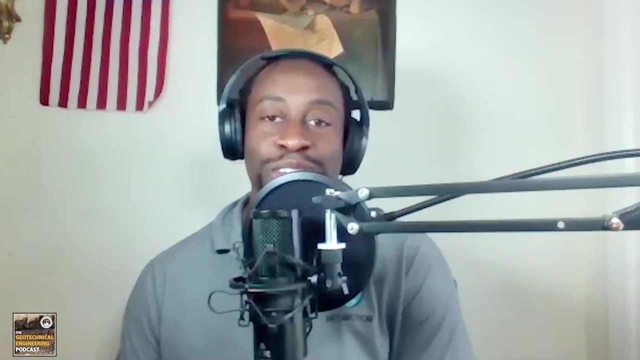 there We should be. our goal should be to work as closely as we can with industry. Otherwise, what's the purpose of what we're doing? Yeah, no, you're absolutely right. I mean honestly, if you're looking at the students that you know they're matriculating an institution and they're 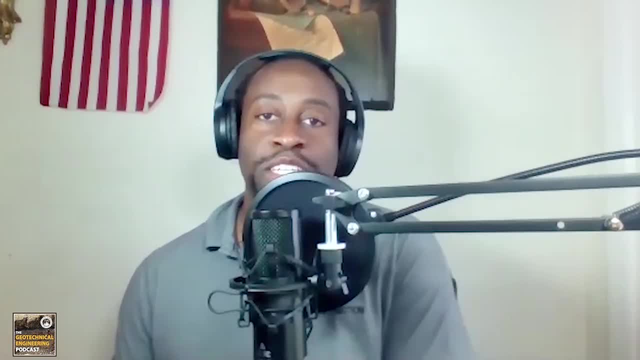 trusting that what they're learning is going to be applicable. So when you bring back you know professionals that are doing this in a day in and day out. it really does help to solidify with their learning, I can think as a grad student. those are some of the lectures I enjoyed. the 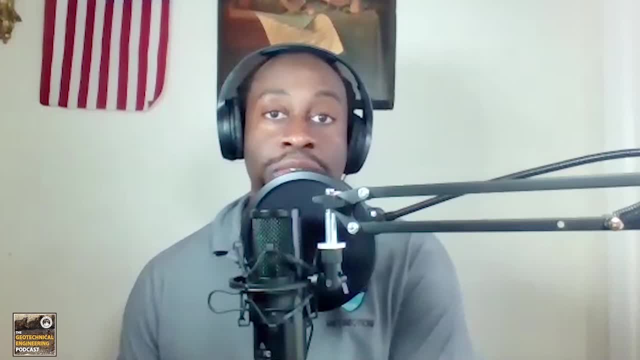 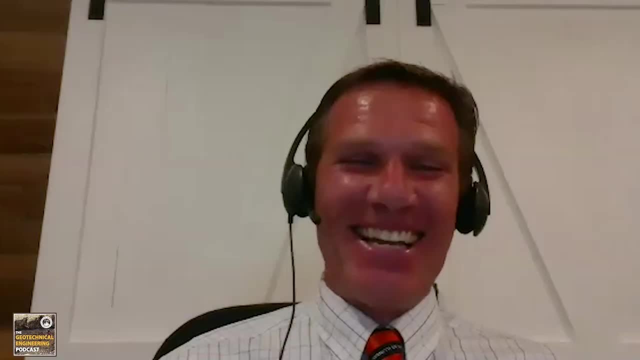 most, or when you heard about a case history or you saw something that didn't go right and how they were able to adjust things in the field. So those are good things. The proverbial handshake is a good thing. Exactly, You know, one of the biggest. 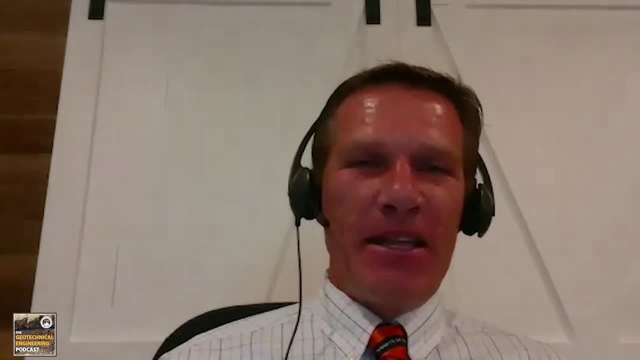 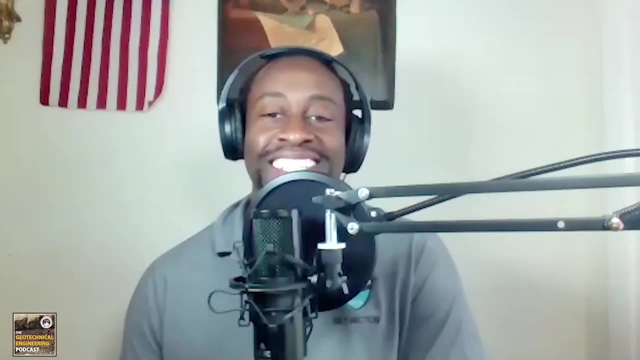 can pay me is that when they tell me the course they took with me was one that they use all the time, that they're always going back to their class notes and referring to their class notes when they're in practice, And that tells me that I'm teaching them stuff that's valuable to them. 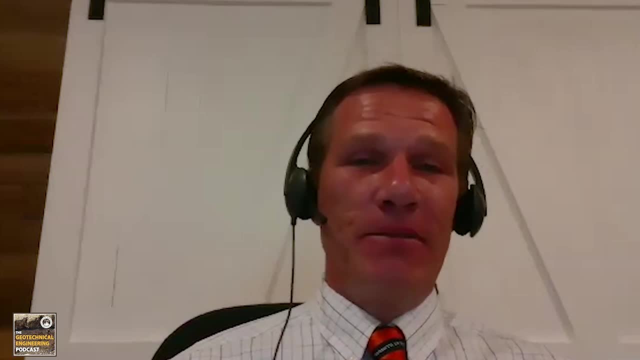 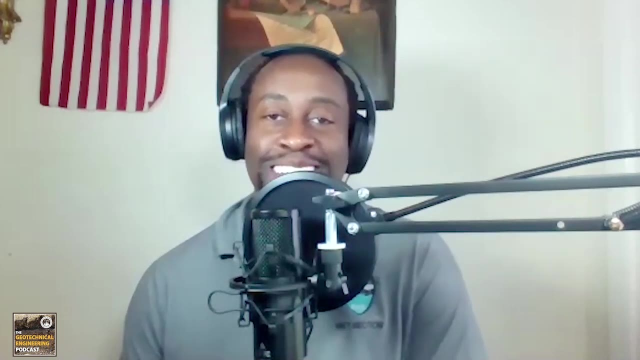 And it's not just, again, things that are going to be stuck on the shelf, Excellent, Excellent. Well, you know, it wouldn't truly be a conversation now if we didn't say something about COVID-19.. We've talked about it ad nauseum at this point, but you know. 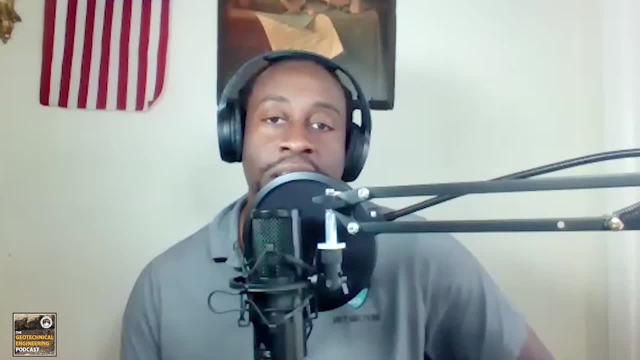 but teaching and researching in this era of COVID-19, I have to imagine that things have changed for you. So what kind of changes have you seen? Pluses, minuses, How are you adjusting? How are you pivoting- People like to say pivot- How are you pivoting at this? 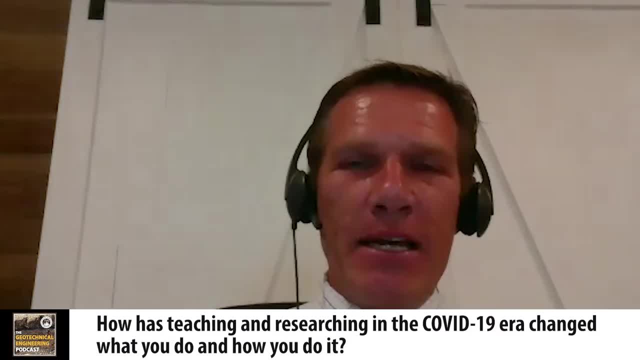 time, So we were really fortunate. at Illinois, You're probably aware that we've been moving a lot of our content, particularly the graduate content, to be available online. We've started offering an online master's program for several of the departments in the grain. 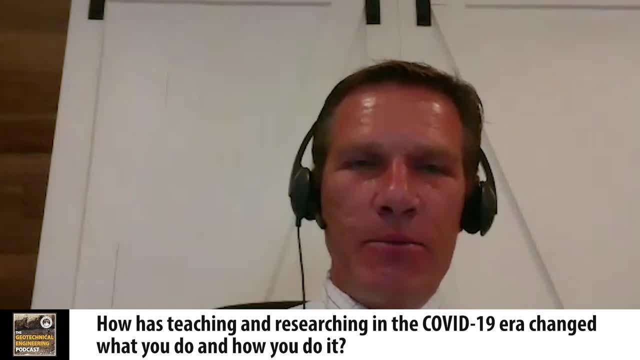 or college of engineering at Illinois And it's been fairly successful. I've had in our graduate courses. I've had up to about a third of the class be online students And I've had students from Asia, not just from Japan, China, from, had one from Australia, had a couple from South America. 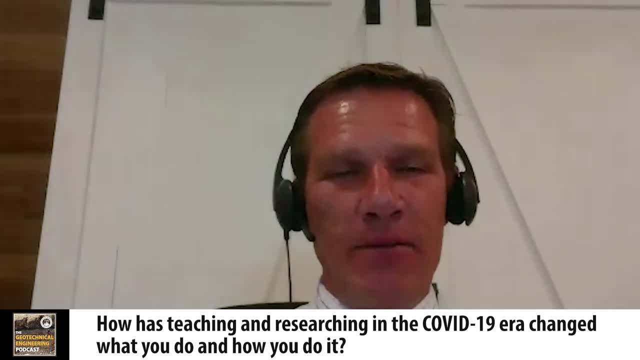 and all over in the United States. So it's it's really kind of interesting. It brings a new flavor. We're still working to the point where it is live. but when you've got students distributed all over the world, it's not always practical to do that live. So we've 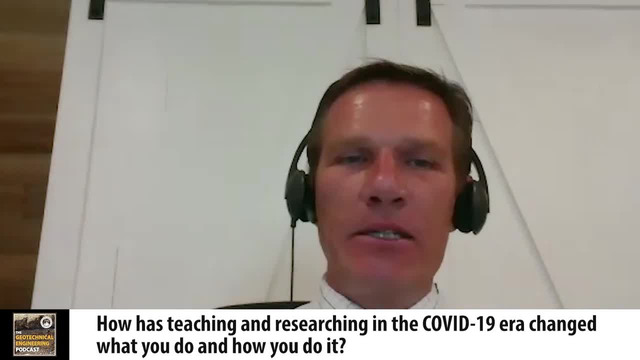 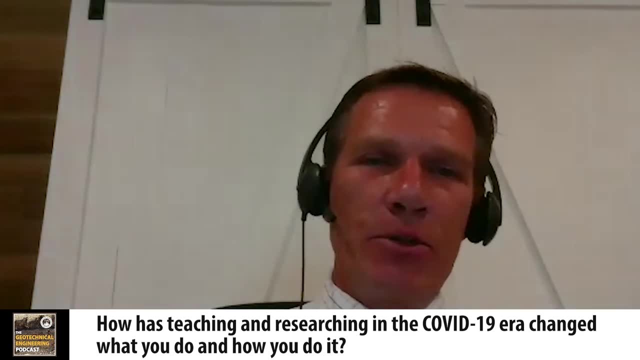 gone with more of an asynchronous approach to in developing this online program. So for for many of us at Illinois it wasn't that difficult of a step to move into the purely online. It was the most difficult that folks had was on the in those really large undergraduate classes. 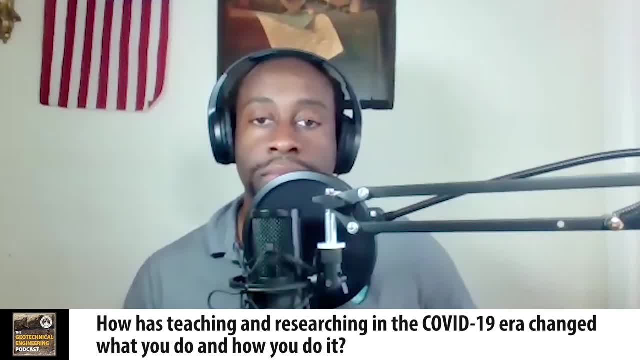 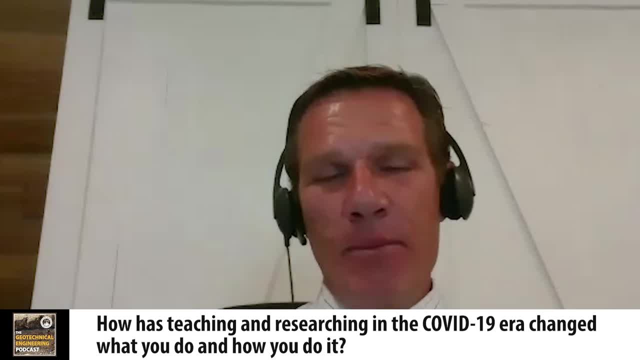 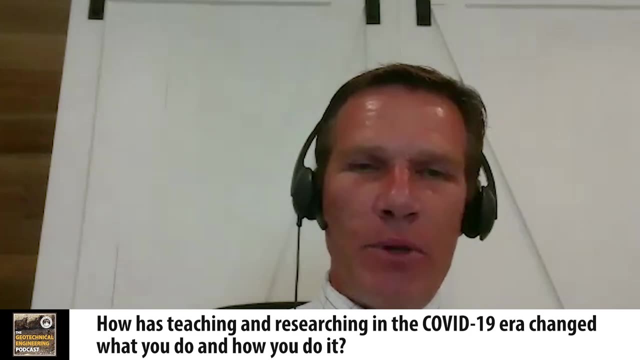 or a geology lab or a chemistry lab. you can imagine that it's just not the same thing. So that's where our faculty had really been striving to provide a meaningful experience for our students. And, going forward this fall, our plans are to have a hybrid system where we have students 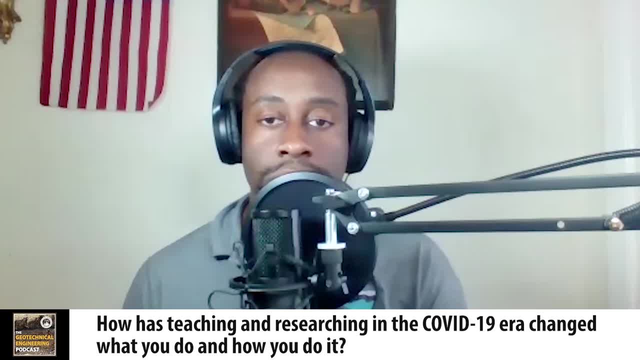 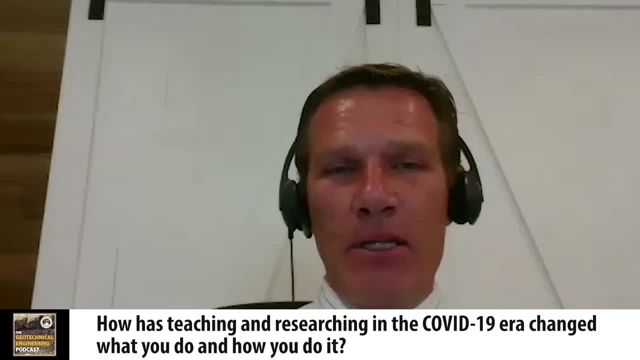 on campus. They are in order to maintain that physical distancing that we have to and to take into consideration the ventilation in a lot of the buildings. they're saying, for example, one-third of the students can go to class on Monday. the next third on Wednesday. the last third on: 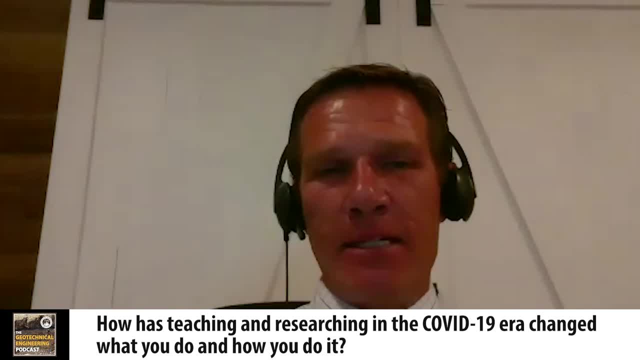 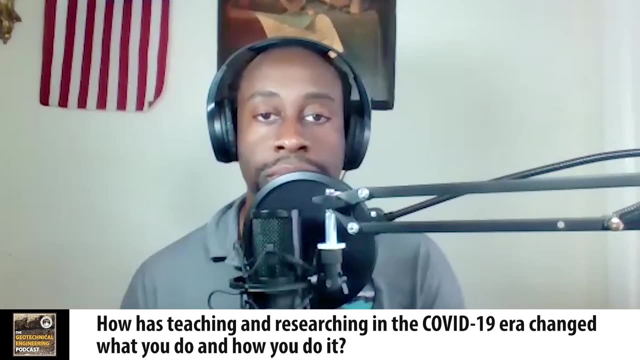 Friday. So we've only got a third of the student body in class live on any day and then the rest of them can do it online. So we're trying to offer more of a mix of live and asynchronous sort of education. So we're still learning, But again, fortunately we were in a little bit better position. 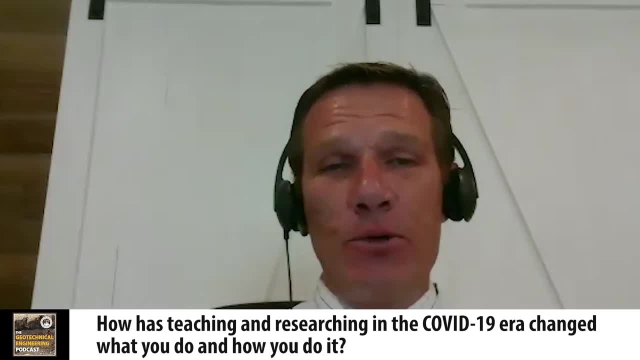 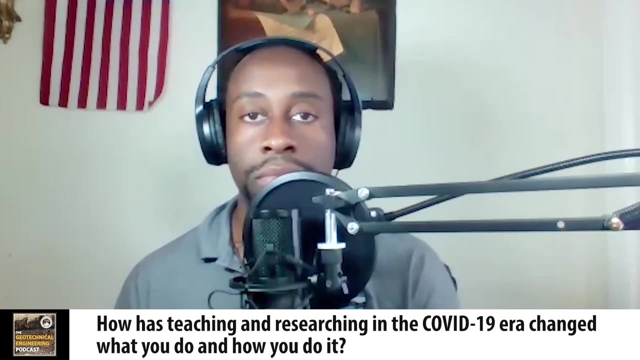 than a lot of other schools to make this pivot to the online education. With research, it's been more difficult because when the university closed down their classes, they also closed down all the labs, So all of the instructional. not just the instructional, but all of the research. 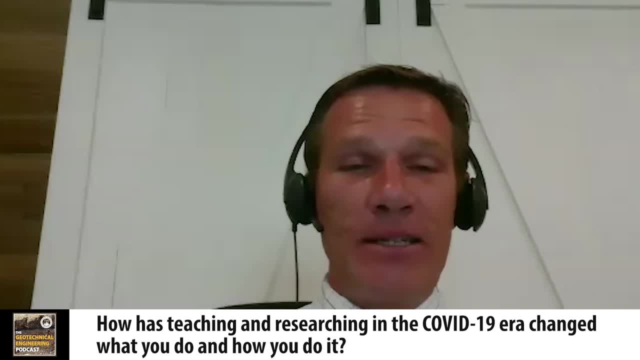 labs closed down. So just now, toward the end of summer, classes are just a few weeks away. We're finally getting the students back into the geotech labs. We're finally able to do some of the field work again. I had students traveling out to UC Davis to use the centrifuge facility. 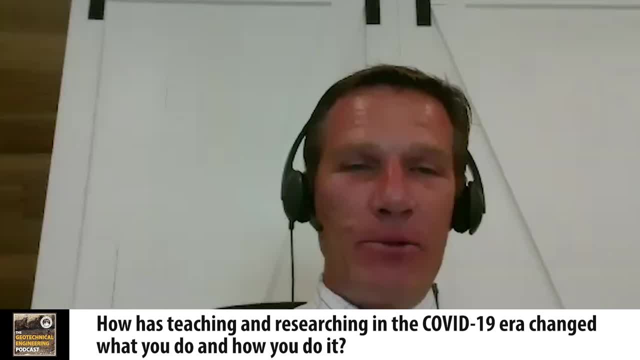 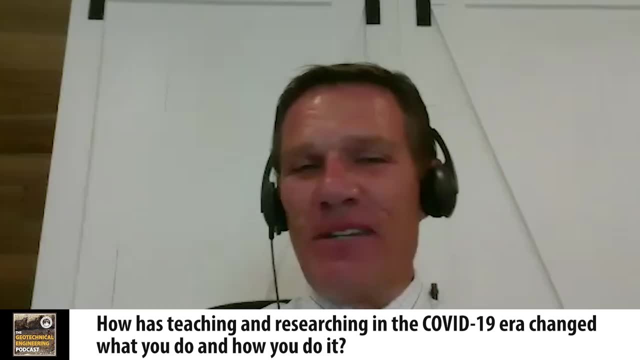 for example, Really Okay, Yes, all of that was shut down and we don't know when that's going to reopen. Wow, So the students' PhD. we had to completely shift gears on what this student was going to do. 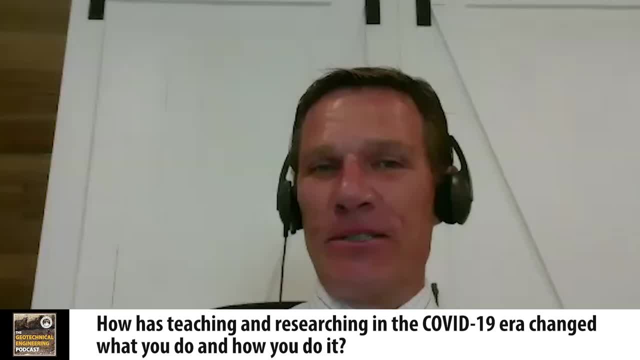 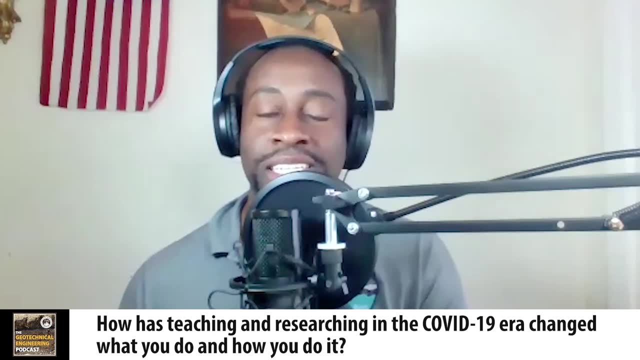 just in case he was unable to complete his plan. But it's planned a scope of war for his research. Wow, And I have to imagine that that's. I'm sure that some of these grants have timetables and milestones have to get hit Wow. 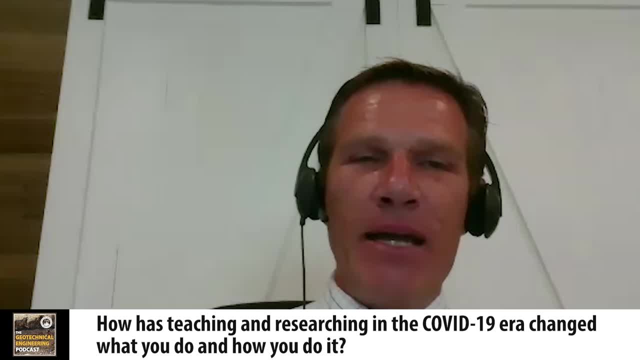 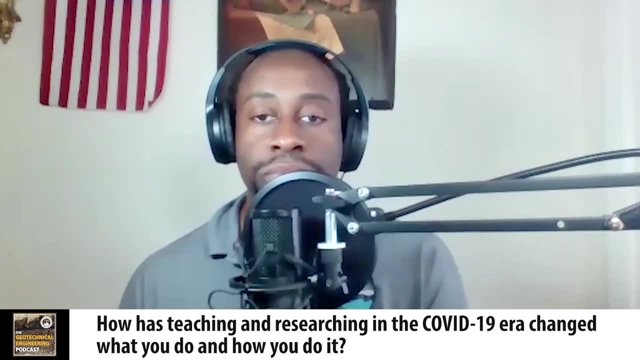 Yes, And fortunately our funding agencies by and large have been understanding of these sorts of things because they're undergoing, they're in the same situation as everyone else, So they're trying to keep deadlines and going from one Zoom to the next Skype to the next. 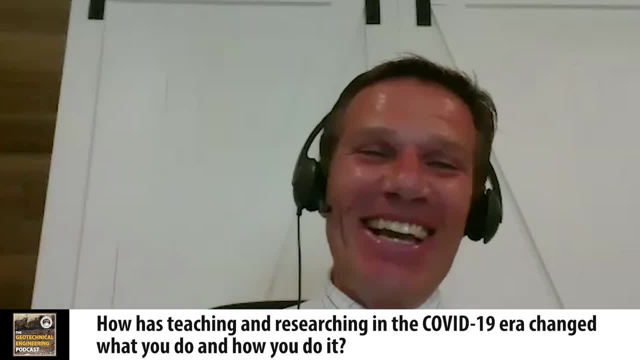 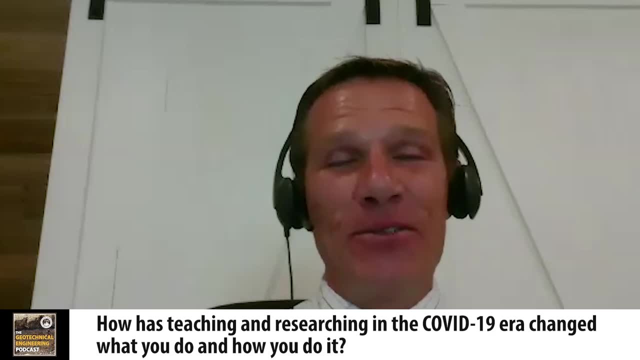 Teams meeting. You know how that is. That's exactly the way: it is Challenging, But it has forced our students to be- at least my students, that's who I've been speaking with mostly- to be more communicative. 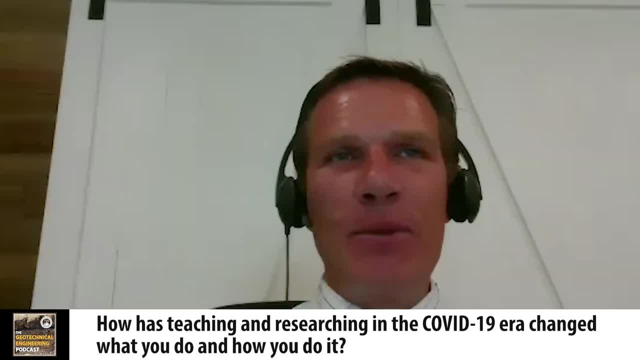 They've been forced to. actually, instead of being able to come to me at any minute of the day in the office, they have to develop their thoughts, kind of develop questions. maybe send them to me in advance so I can think about them, And then we, you know, we have a set time where we meet for a 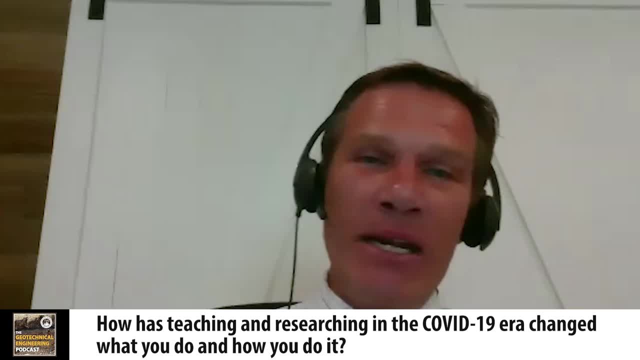 set amount of time because, just like everyone else, I've got another meeting coming up right after that. Yeah, So they really have. I think it's been a nice experience for them from that respect- not overall, but from that respect from the point of view of having to really focus on communication and developing their thoughts. 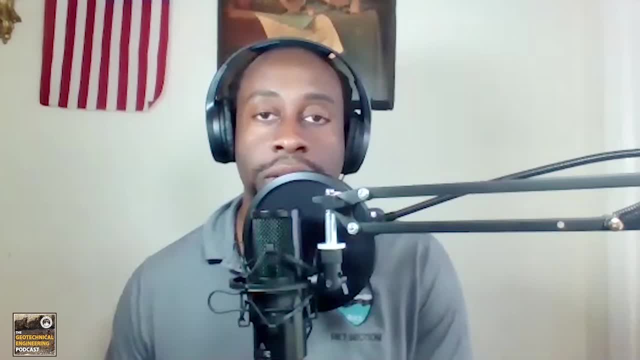 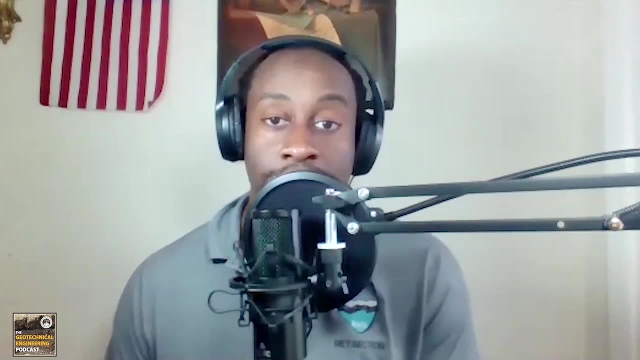 So pluses and minuses, just like with everything, Got it? No, it's definitely key, I wonder. I think that you know I've seen one, One of the challenges whenever I have to present. now, it's all you know, it's virtual. 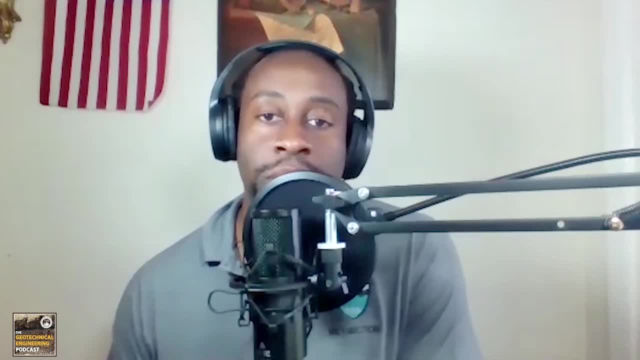 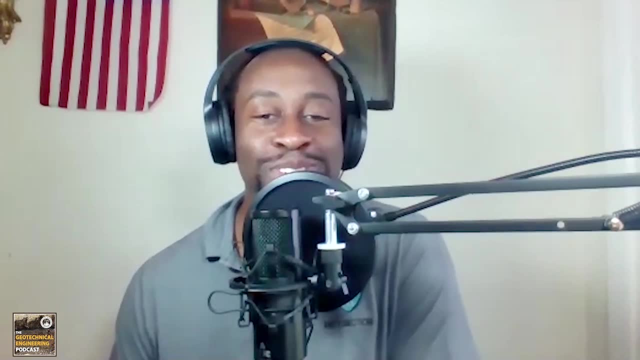 So you're talking to a computer screen, but I envision it as a professor. It must be a little challenging. You don't really get energy back from the students. You can't tell if people are checked in or checked out. How are you resolving that? 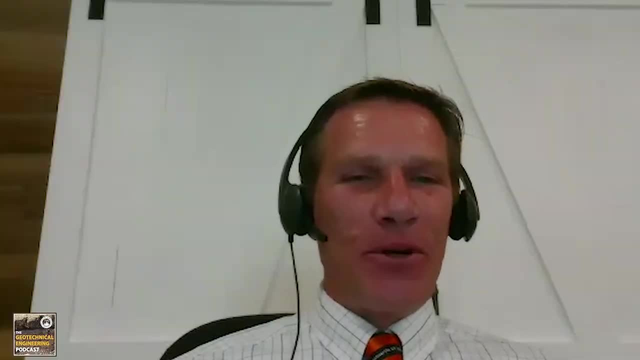 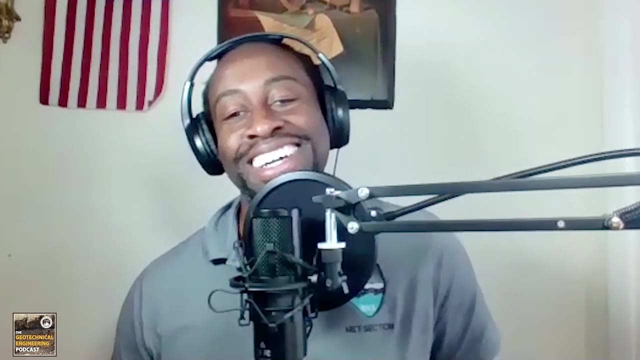 The end of the semester after we closed down following spring break was really odd because I talked to an empty classroom, like a lot of our faculty did, Wow. So at first the echo was really, really bizarre, Not having students in there to kind of absorb sound. 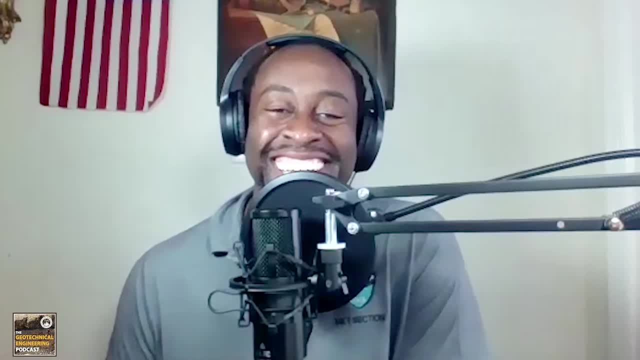 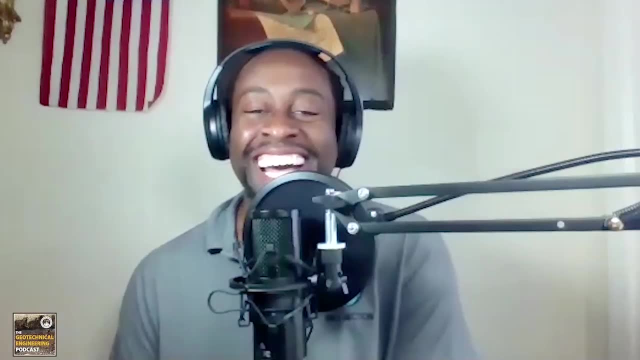 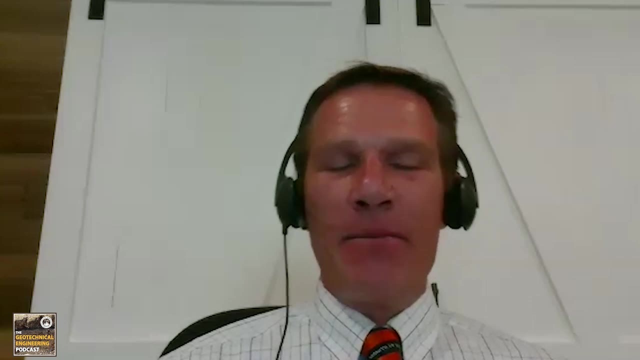 Yes, All the classrooms echo. You can clearly hear the instructors in the next classroom teaching. Oh my goodness, So you're trying to talk over the next person. But what I tried to do then to make up for that lack of direct contact is I had immediate. 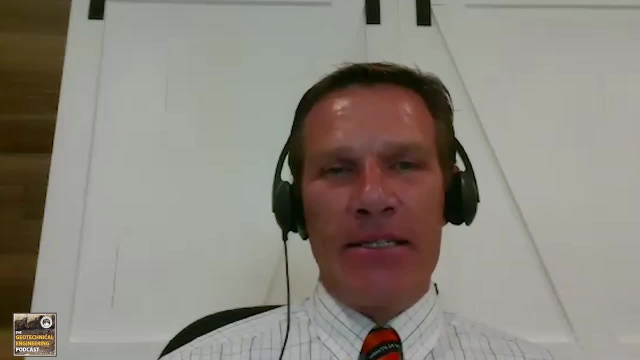 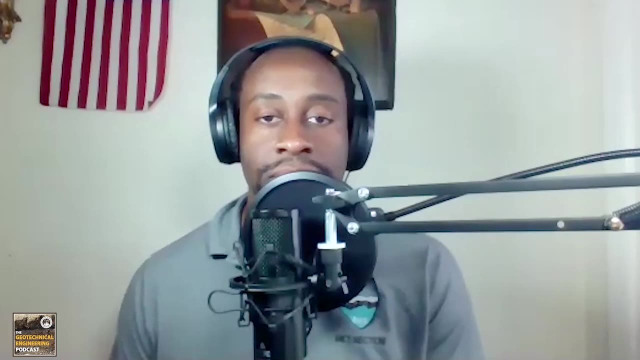 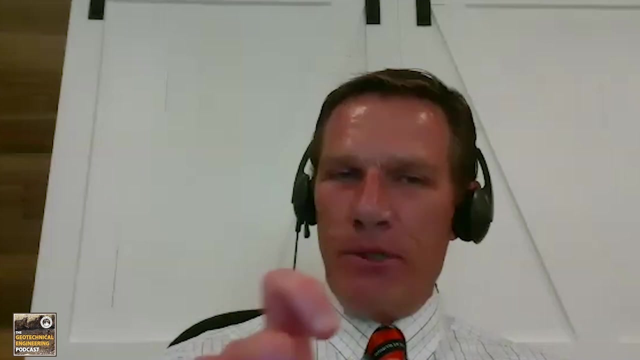 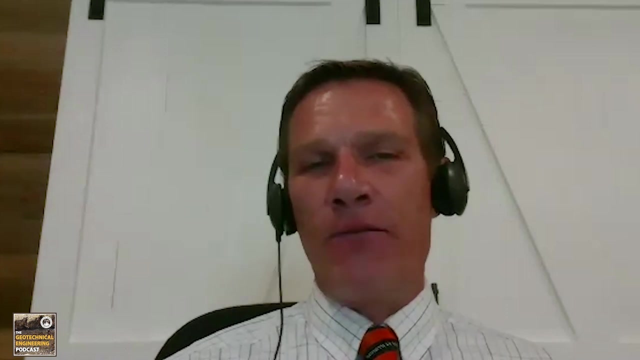 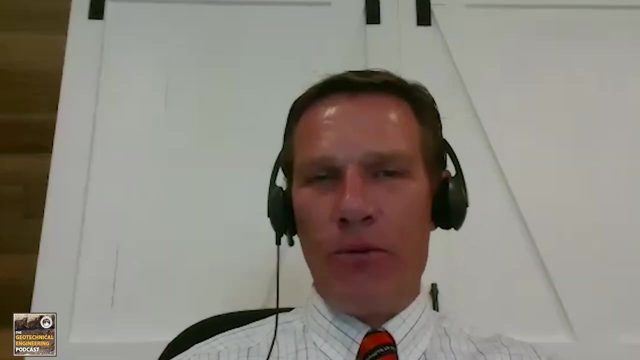 Our system uploaded the online content or the virtual content within about an hour after the lecture was captured. Okay, So there than the following hour. I had a zoom session with my students, So a discussion session essentially, where we could walk through. So I open up the presentation and we kind of walk through different points in there and I would try to highlight certain things and then allow for more question and answer. that it made for more work for me because I had to for every hour of classroom time where I do both the lecture and the question and answer. 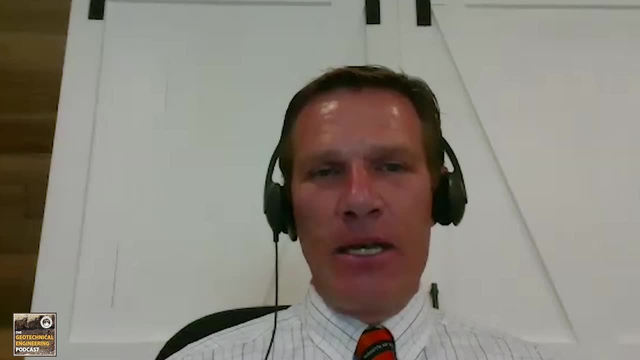 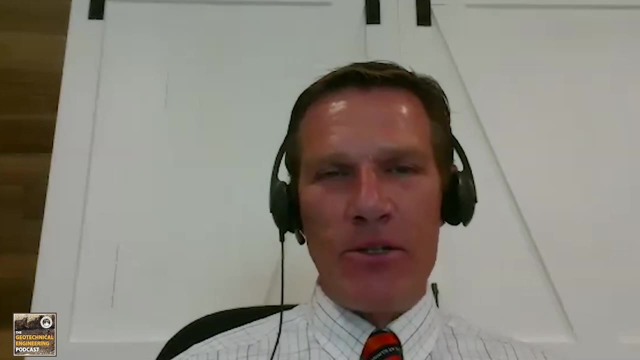 Now I had an hour of lecture and an hour of Okay, And then I held separate office hours so that I could go through homeworks or meet with students individually in that fashion. So it was a little bit more time consuming, but I think we everyone seemed to make the best of it. 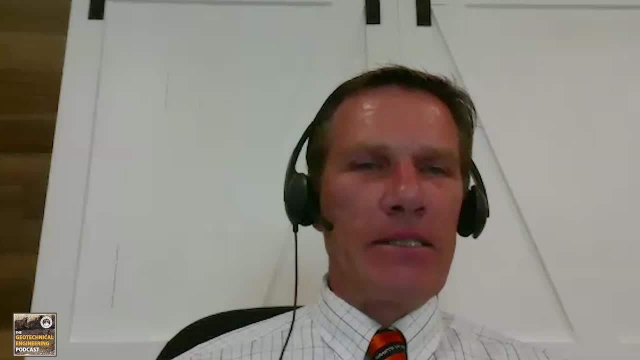 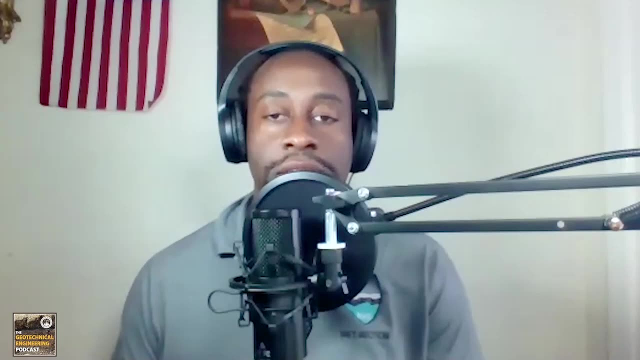 And I had a good, good attendance at both office hours and the question or, excuse me, the discussion sections. Most every time That's a good sign. It's a good sign. Yeah, It's a little different, but but again everybody was the good part of it was everybody. 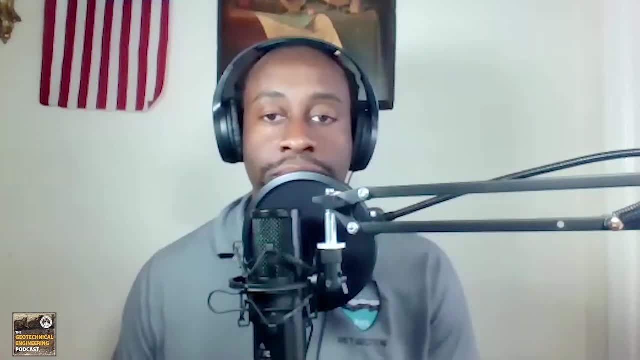 Learned how to be flexible. Yeah, I'm not terribly flexible person, I'm not the biggest proponent of change, but yeah, I realized that that is that that's the only constant. as much as that is a cliche, It certainly was the case last semester. 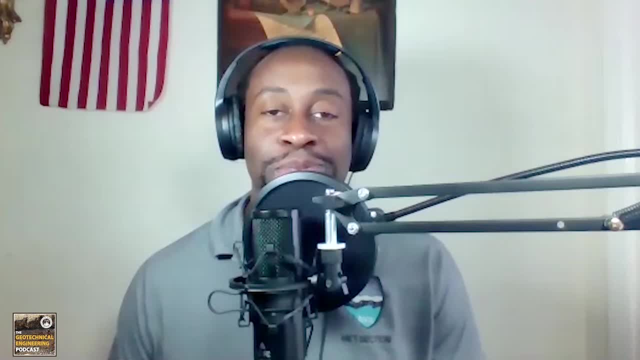 It's going to be the case for this coming semester. Yeah, you're absolutely right. There's a. you know we in the and, as a design professional, one of the challenges we often hear people talk about is, you know, work life balance. 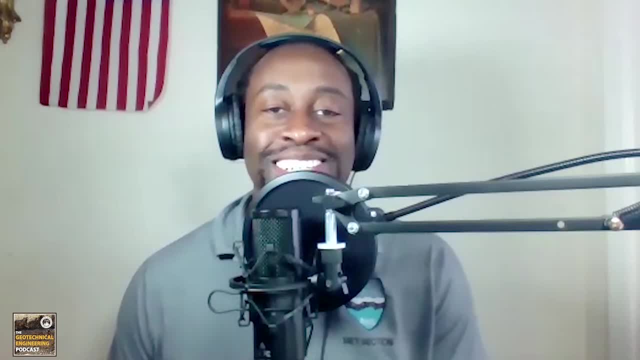 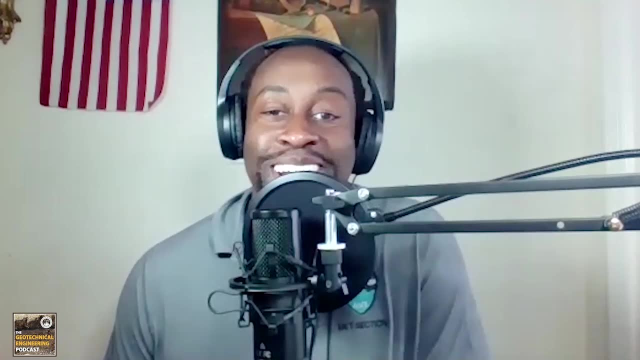 And I've talked to some of my mentees over the past Months and they say all it took was a worldwide pandemic for you to start thinking about. you know, work life balance a little differently And the reality is we find a way to make it work. 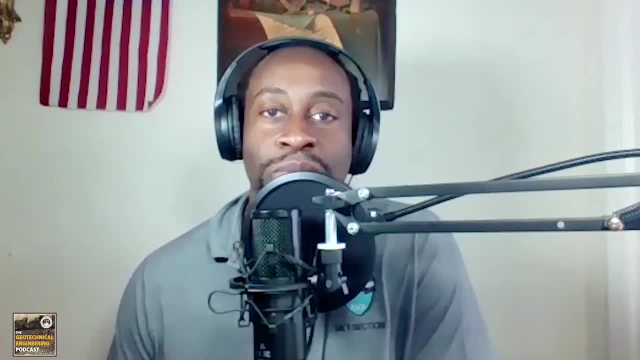 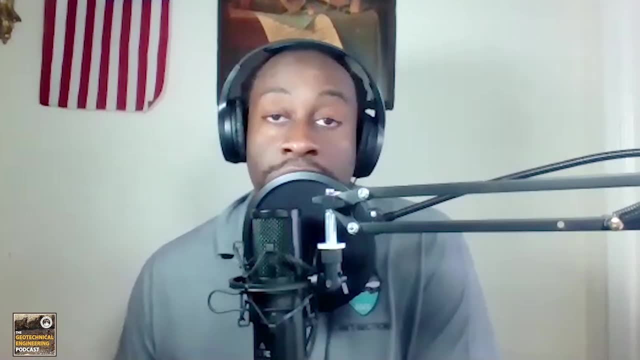 And the same thing in the in the. as a professor, it's like we have to find a way to still be able to instruct the students. So that's really awesome. That's really awesome. Well, I look at your bio and I look at your history and what I know of you. you you've won a lot of awards and honors for your research. 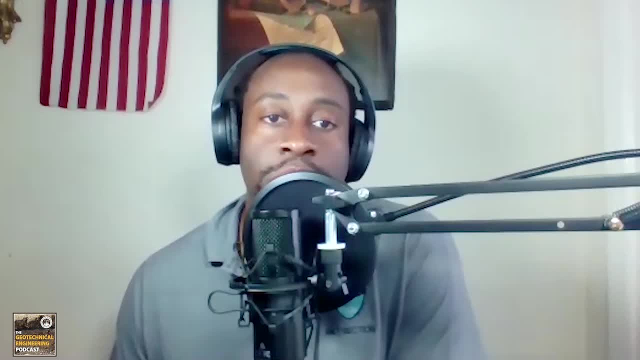 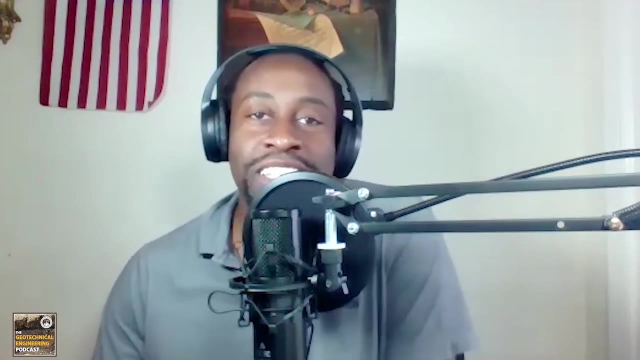 Uh, that's really been practice related and your teaching accomplishments, And one of those uh focuses has been on resilience. Yeah, Yeah, Residual strength of liquefied soils. Can you tell us a little bit more about? I mean, of course, if it's, if it's, you know, top secret? you know don't share that part, but can you, can you share some of the uh updates and some of your latest developments? 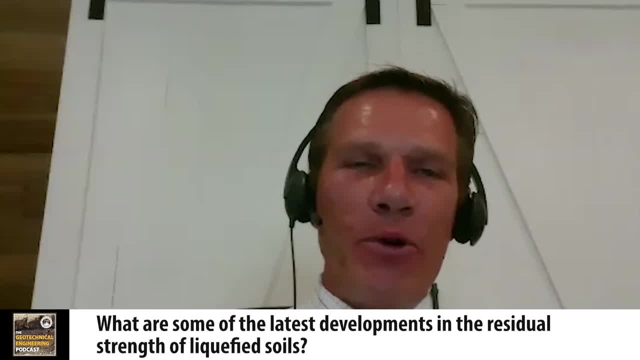 Sure. So, up to this point, everyone, when you think of earthquakes and liquefaction, you think sands, And so most of my work up to this point, and some of the things that had been recognized, had been on how sands behave during earthquakes, or 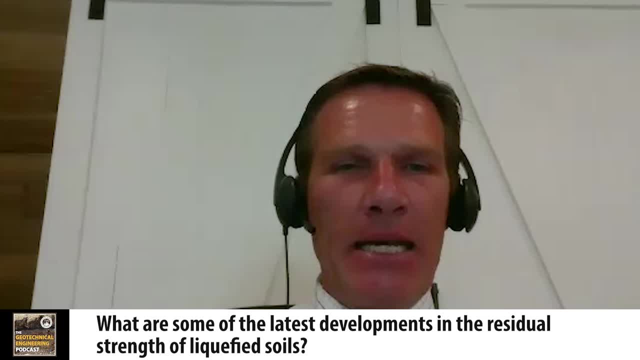 Yeah, Under, Yeah, Big slopes and and in within dams or underneath dams. Yeah, Yeah, Yeah, Yeah, Yeah, Yeah, Yeah. Now the profession is realizing and it's. it always takes us a little bit of prodding to kind of recognize all of these different aspects of the same problem is that silty soils may be subject to the same sorts of things. 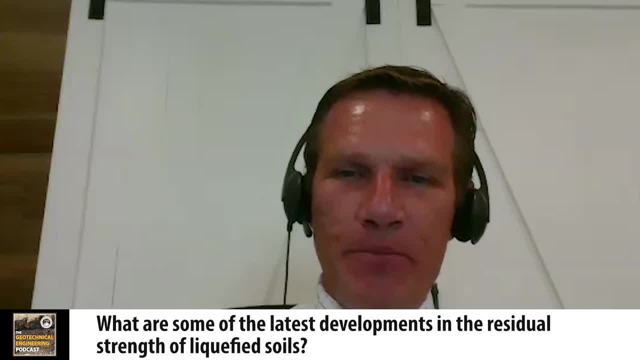 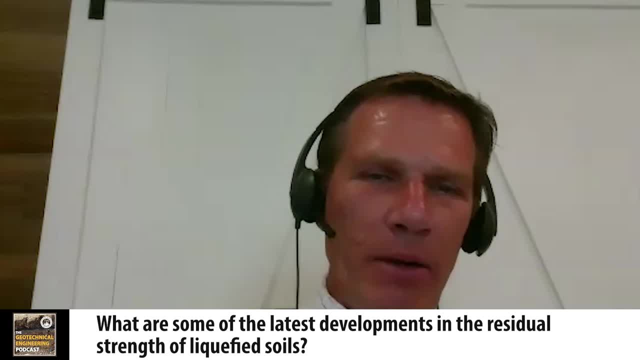 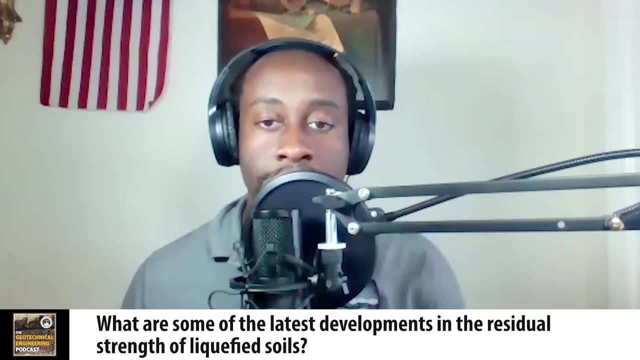 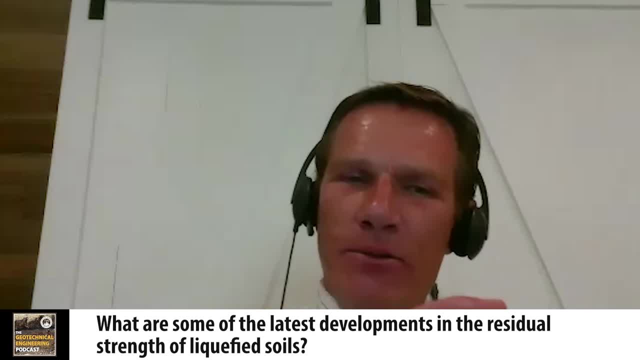 to cyclic softening. and then how do we take those ideas when we and move from natural soils to anthropogenic soils, the, the tailings, the fly ash and all these sorts of man-made materials that aren't exactly natural soils but they're not exactly perfectly round spheres either, that. 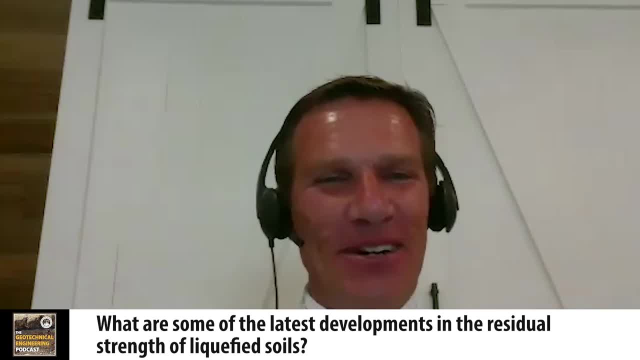 the physics guys can get into and really take over how things behave. so how do all these concepts for sands apply to these, uh, man-made materials or industrial made materials? and then, given that we're now transitioning from sands over to more fine grain and clay soils, what's the best way to? 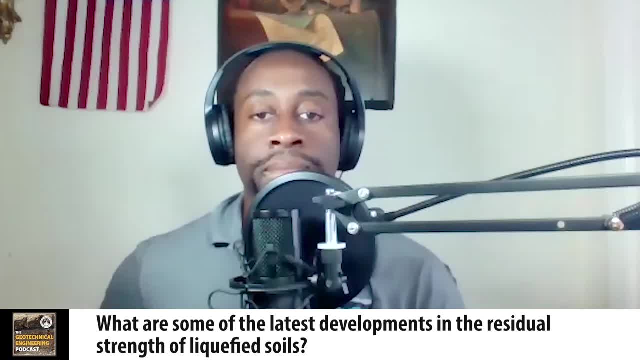 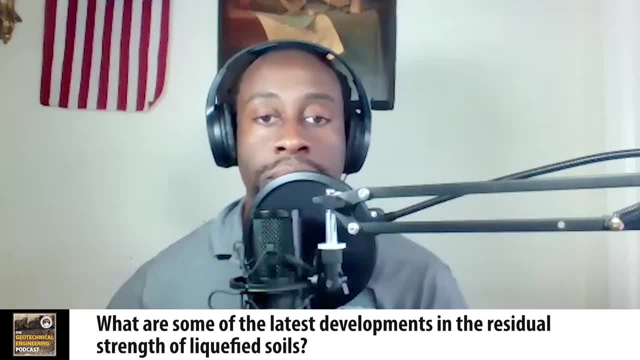 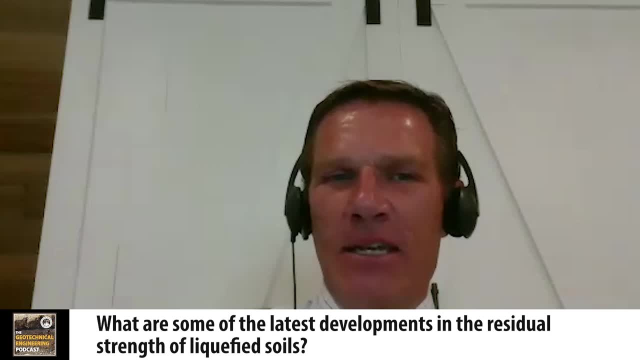 laboratory testing and when you're in this transition in the silty zones, do we go lean toward sand or do we lean toward the procedures that we have for clays? and so it's really, again, that's more practice related, but it's a really critical question because you're talking about 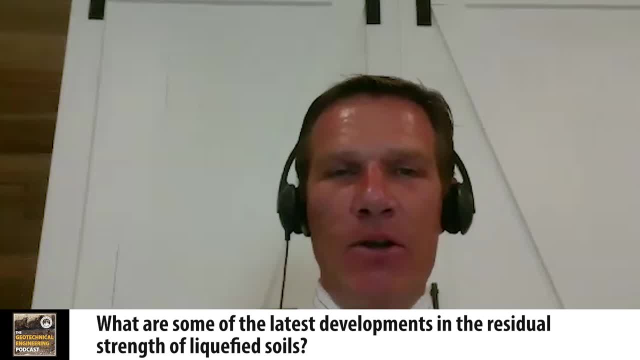 you know the case of tailings dams. you've got hundreds of or tens of millions of cubic meters of this stuff being held up by sometimes very thin shells of stable material and it's been- there's some been some really high profile failures of those sorts of structures in the 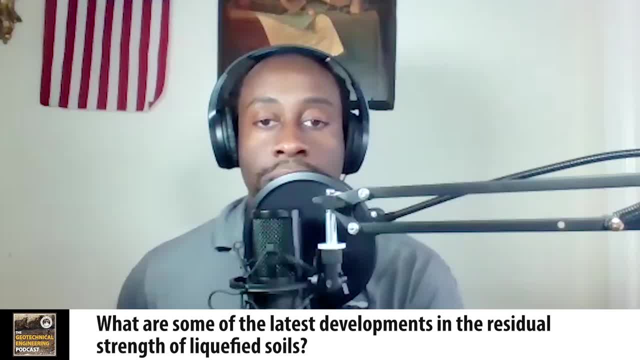 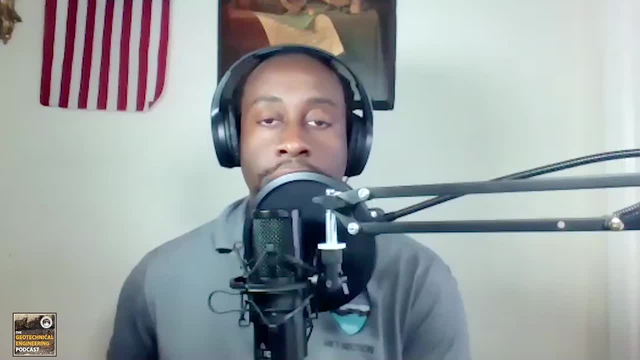 last five or six years, indeed, indeed. so how do we, how do we then take these concepts and apply them to practice, and what's the best tools to do that got it and what got you interested in that you? you had the- somebody asked the question and you started to delve into. 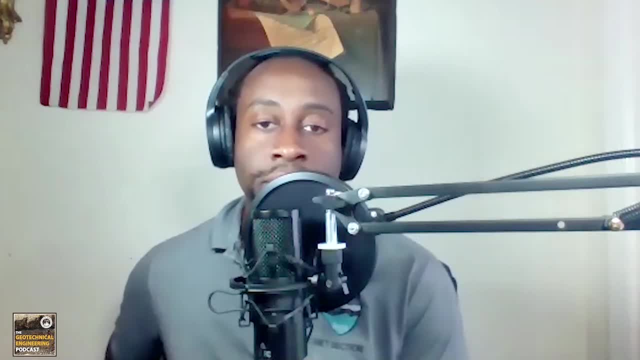 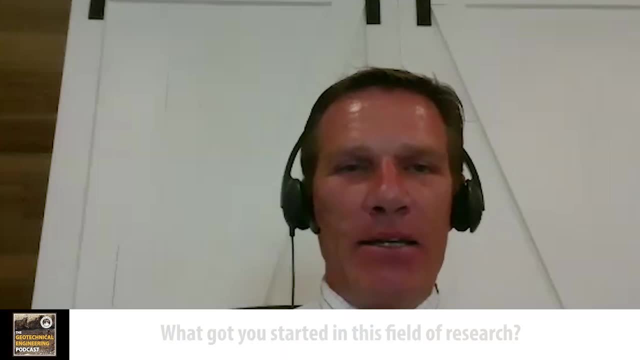 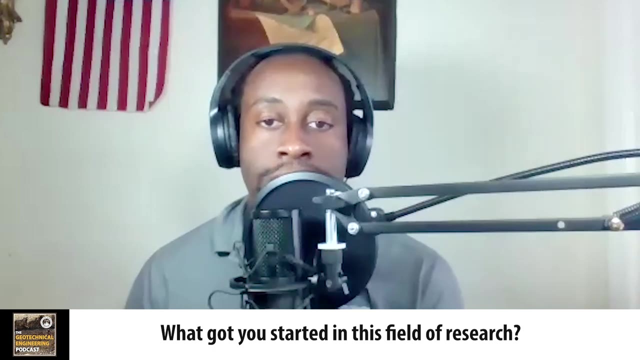 it an opportunity or a specific grant you're going after. i mean, how did you so? it was from the beginning, early on. my return to illinois for a phd coincided with the beginnings of the three earthquake centers across the country, so historically it was always centered at uc berkeley. 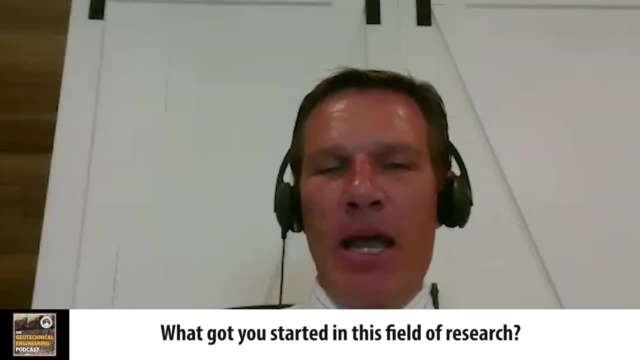 and that was the pacific earthquake engineering research center. and in the late 90s nsf funded two additional earthquake centers, one's headquartered at illinois, the mid-america earthquake center, and one headquartered at rensselaer polytechnic institute, the multi-multi-disciplinary center for. 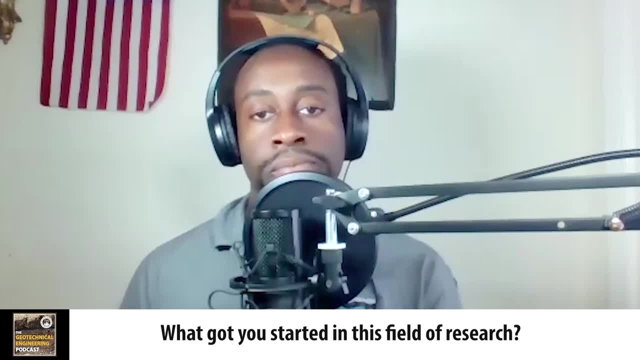 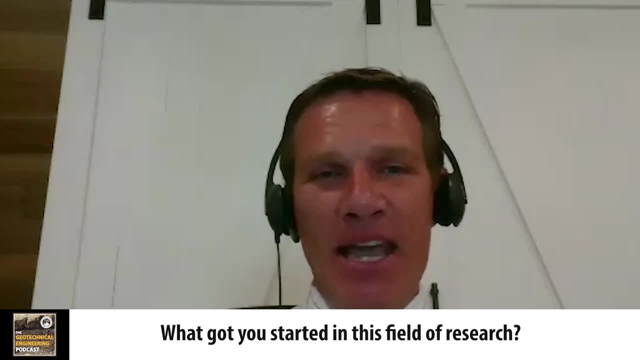 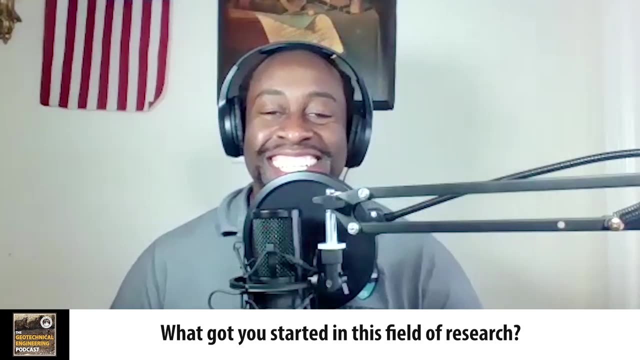 engineering research mc, and at when that started up i was asked to actually, my advisor called me up and said: hey, do you want to come back and work on a phd? i was in the middle. i was a practitioner, just like you and i on a projects. i was actually away from home at the time on a project site. 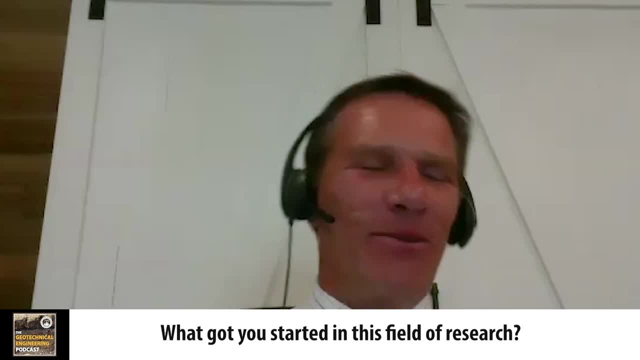 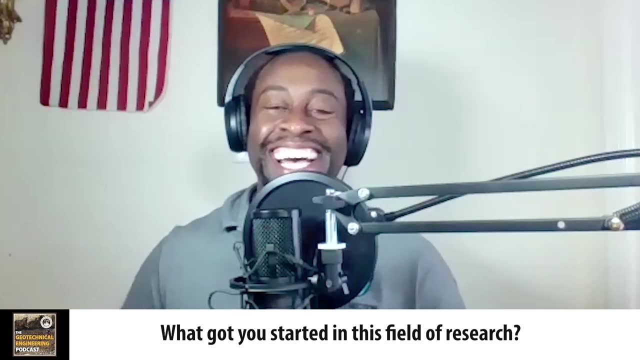 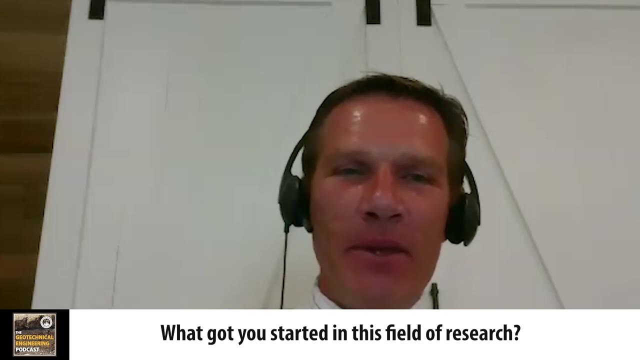 and i said, well, yeah, i give it, yeah, the door's open. yeah, maybe one day i want to teach. why not, why not give it a shot? and so that's it's. it was essentially just the door, right door, opened at the right time and allowed me to kind of 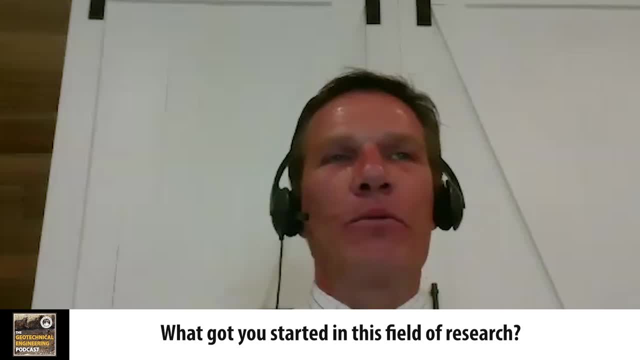 expand my skills and and develop or get the skills that i needed, that i could open more doors in the future. and what i mean by that is without a phd i wouldn't be able to teach really at the level that i might want to teach at one day and i really didn't have a desire to go into academics at the 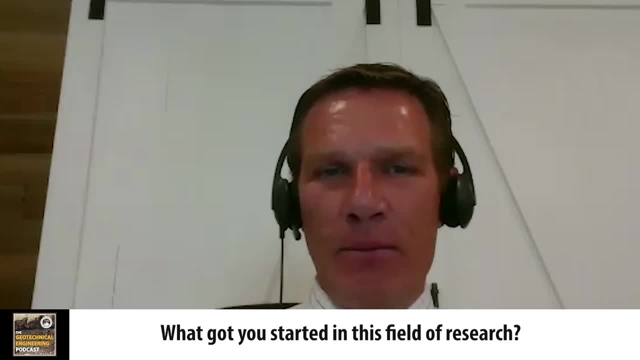 time, but i wanted to have that option later in my career. that's awesome. that kind of started me in that direction and it has really just kind of evolved, uh, along with my- you know, along with me and everyone else, my interests have evolved to some extent, but they've also kind of stayed focused on this liquefaction problem and 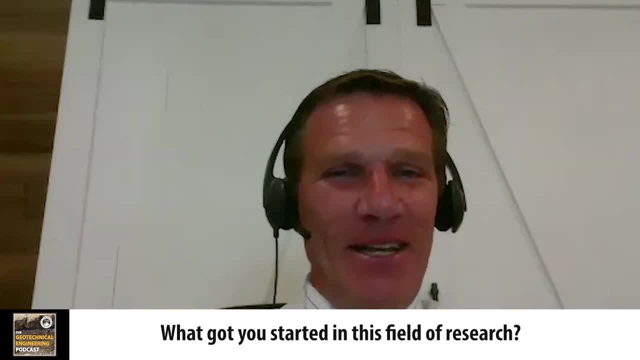 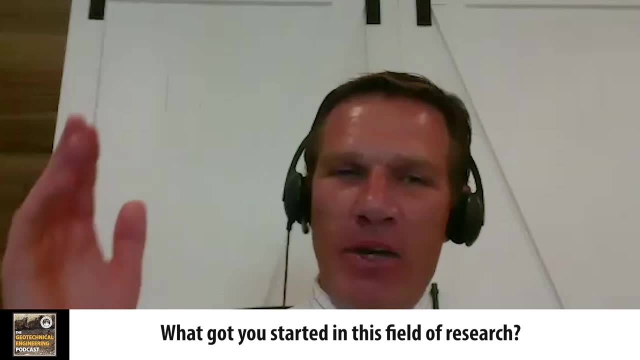 the problems that we apply it to have evolved in this case. so one of my colleagues from when i was working on my master's degree called me up one day and said: we've got this problem with the tailings dam, and this was 15 years or so ago and that got me interested in tailings dams. the interest in 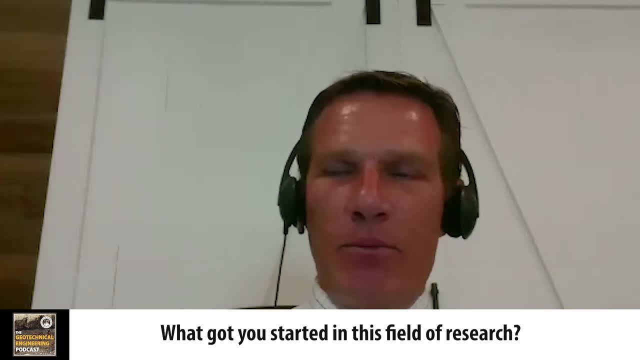 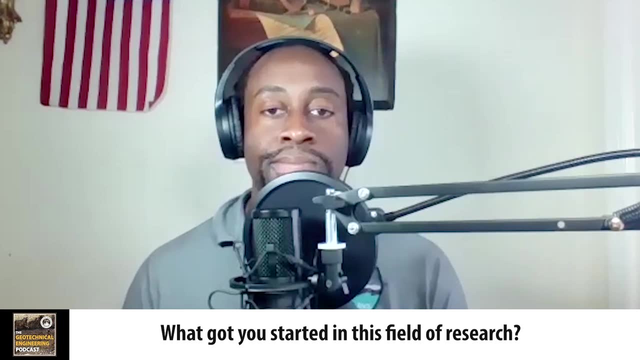 tailings dams and the interest in tailings dams started in practice and it was problems that i got thrown into as a practitioner and i didn't have the answers to those problems that we had to answer. and you run into those sorts of things all the time that, yeah, that there's the line blurs between 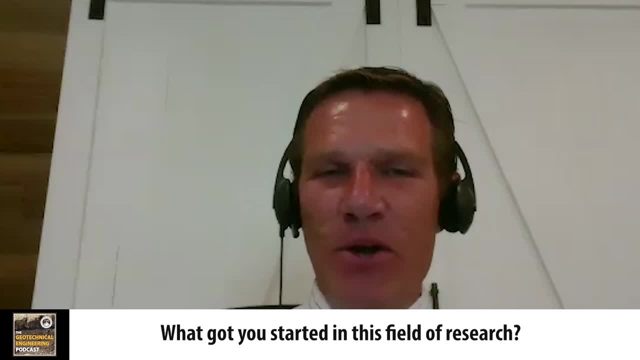 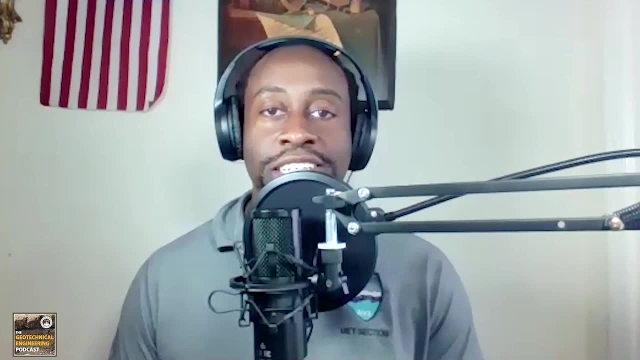 practice and research at times, because we don't always have the answers to the questions that we're trying to solve now. you're absolutely right. i think that one of the biggest uh challenges, challenges, one of the biggest eye openers when you start working on a tailings dam is the fact that 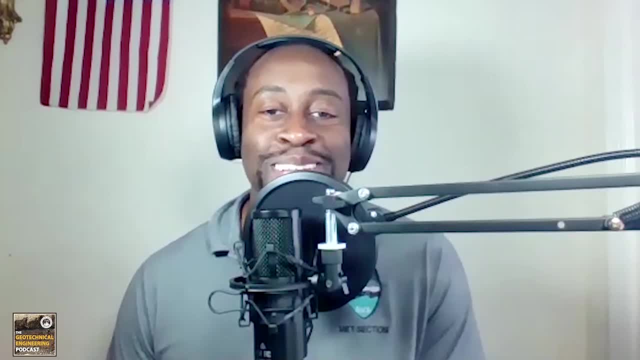 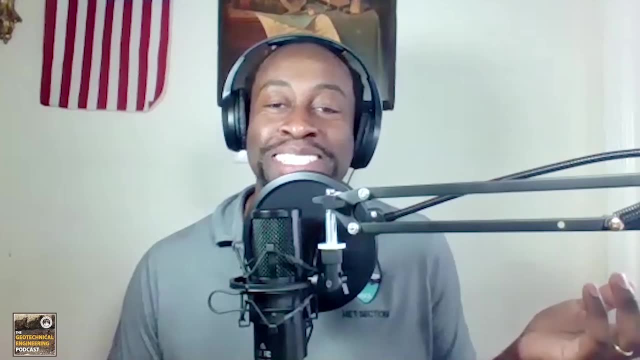 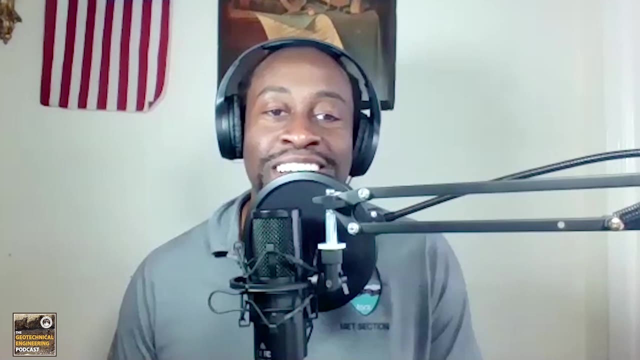 as a professional is, you know you don't always have the given information. so what am I supposed to do with this equation? I don't have any other given information. it's like, yeah, you have to go and drill, or, it's right, push cones and you have to get those parameters. that's great, and you know when you start. 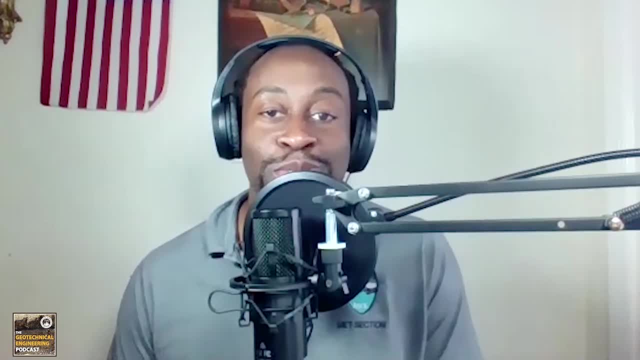 to think about static and seismic liquefaction. you've been studying this for 25 years- quarter of a century. that's quite a long time when you think about the research that you've done and you think about the different aspects of liquefaction. now we have listeners that are from folks that are in college and 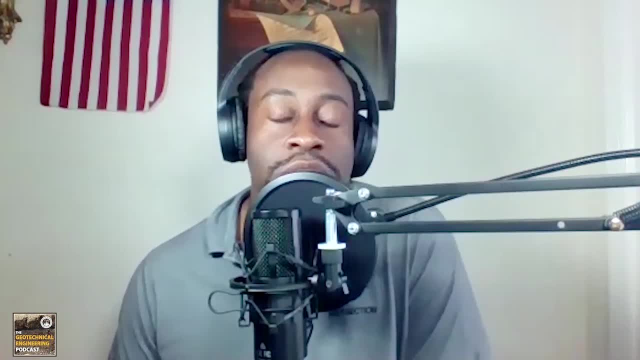 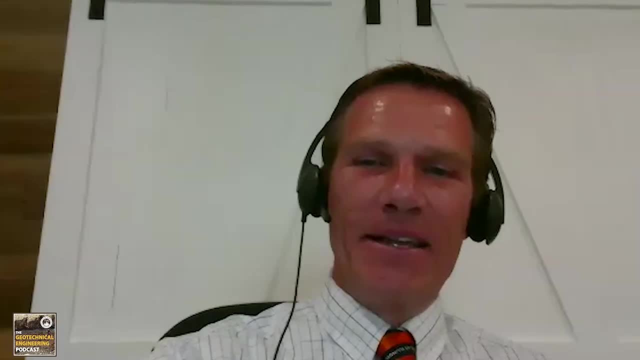 in grad school all the way through to professionals. but what are some of the aspects of liquefaction that geotechnical engineers need to think about? I know you could talk about that for five hours, but I mean, what are the things that come from a high level that come to mind? you know, if, if I could boil 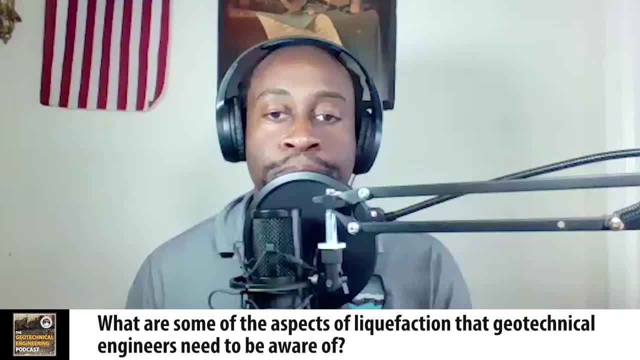 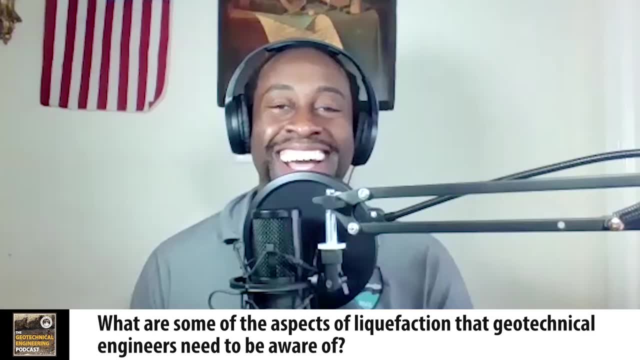 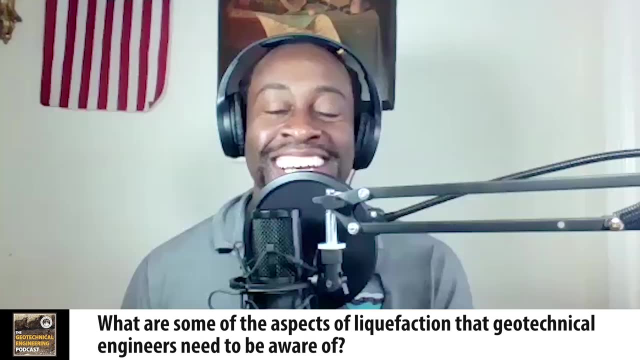 it all down to just one statement: okay, that soil liquefaction is not a magical behavior. Wow, I once heard it term soil liquefaction because it the. the engineer who mentioned that is a practitioner, uh-huh, and he mentioned that and I just sort of gonna laughed because I thought it was hilarious, because a lot of people do. 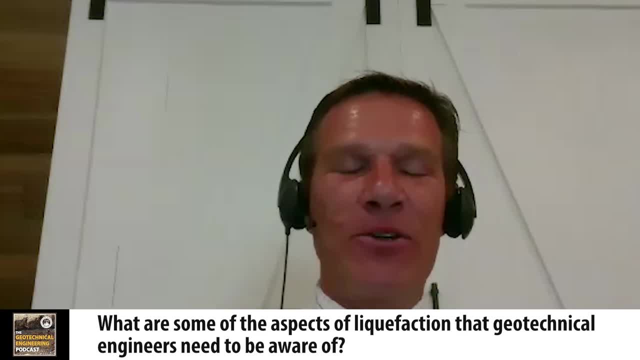 still picture it as a black box or some kind of magical behavior. yeah, and it's really not. it's just soil behavior. it's just stress strain, volume change. and if you understand stress strain, volume change of soils, you can understand liquefaction in all its different forms. 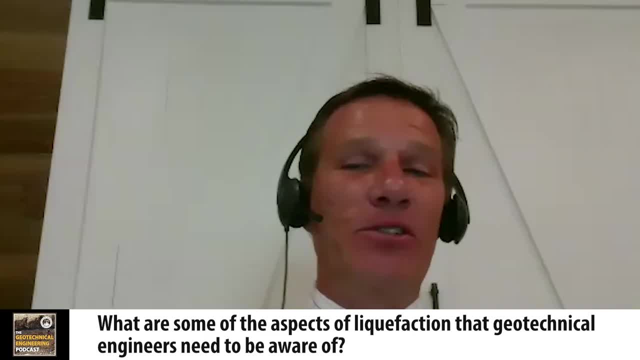 you know, you understand those things. for water pressure, effective stress, shear strength, reconsolidation, you've got a lot of the problems covered, whether it's a slope stability problem or a bearing capacity problem or a pile capacity problem or settlement following liquefaction, you've got all those. 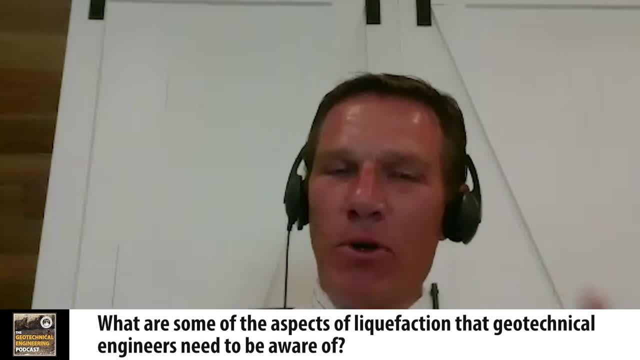 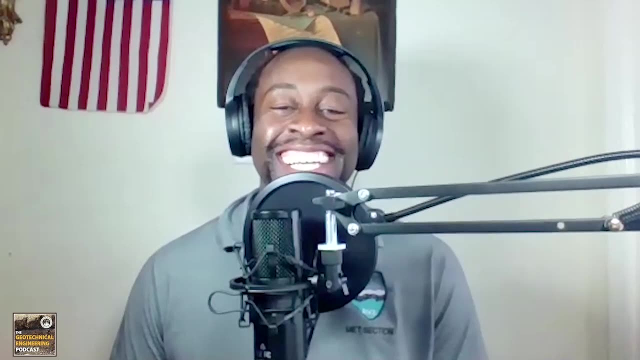 problems in terms of your basic soil behavior cross and and there's no need to think of it as some kind of separate magical land that very few understand understand and very few think is real. It's just soil behavior. Awesome, That's a great way to put. 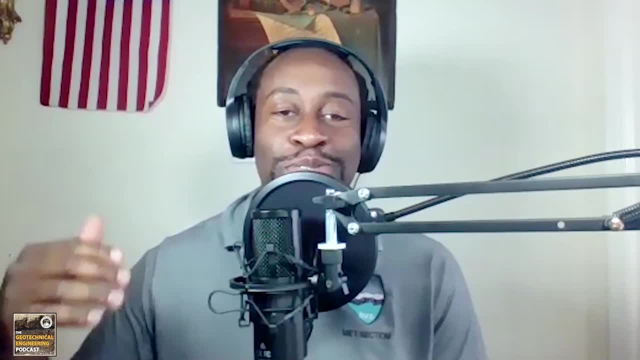 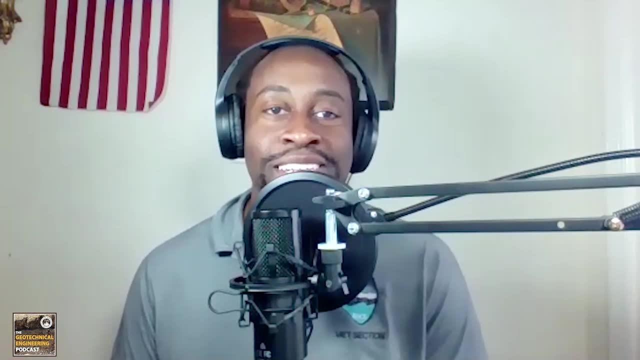 it. I mean, that makes it a little less intimidating for the younger engineer that says, oh, I have to, you know, have to go back to my integrals. How am I going to figure out this solution? But you're right, It's the behavior of the soil and the soil is doing what it does. 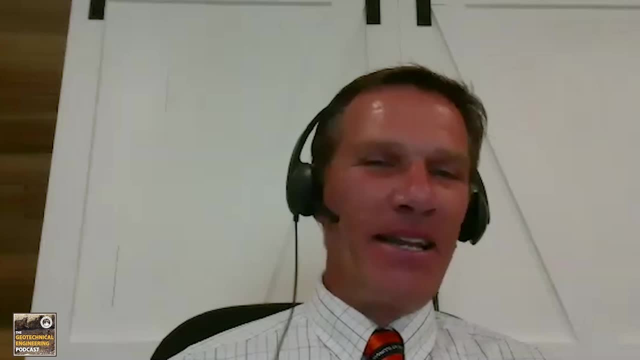 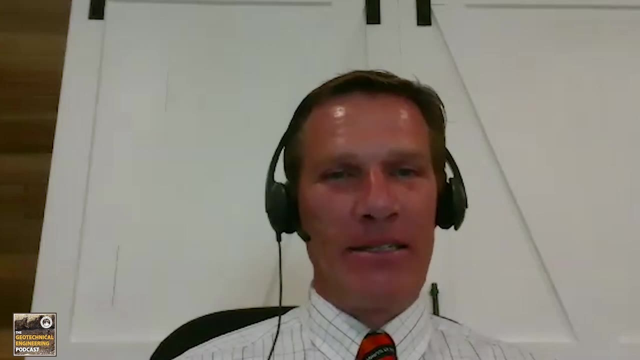 right, That's great. That's great, And that's what I try to teach in my classes- is just understanding the basics of soil mechanics will take you a long way in practice. That's great. That's great. And when I think about your career, you do a lot outside of the 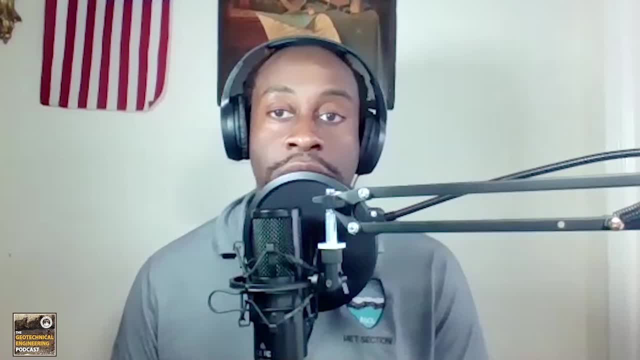 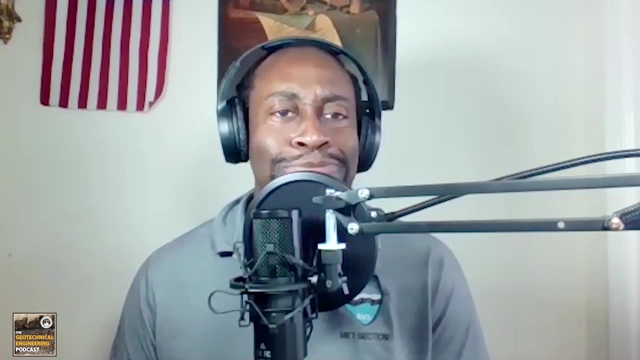 classroom. You know you're a part of a number of professional societies. I won't name them all, but I know, of course, American Society of Civil Engineers, the Geo Institute, the North American Geosynthetics Society, Seismological Society of America and a lot more. How do you factor in? 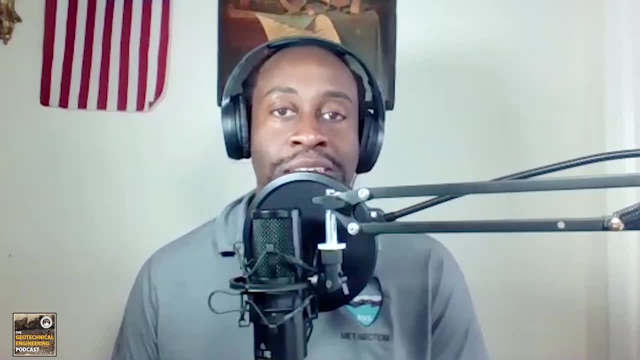 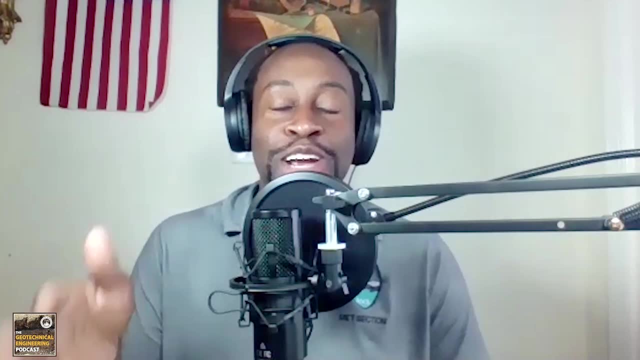 time to do all that, Plus your research, plus teaching, plus handshaking with the professional. Like, how are you, How are you doing If you have extra hours? that sounds like magic, Please share. But seriously, how do you do it all? 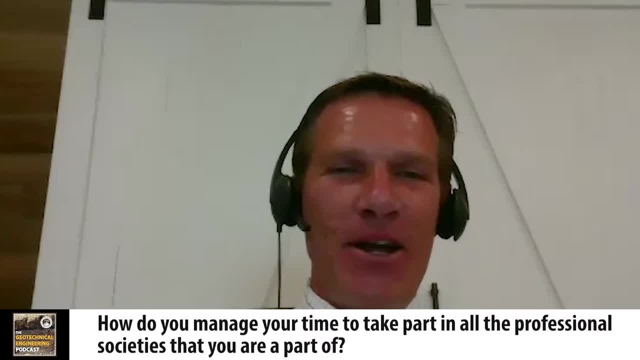 I wish I had an answer to that because I still, you know, as you said, I've been doing this for a quarter century or so and people have been doing longer, People have been doing less time. I don't know that any of us have figured out how to properly manage our time. I know I haven't. 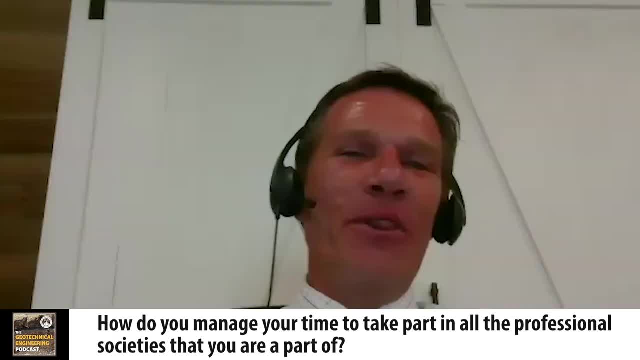 Yeah, me neither. So you know, like you, When it comes to deciding which ones to do which activities to participate in it, I really look at it the same way I kind of look at research is: how can I best use my limited 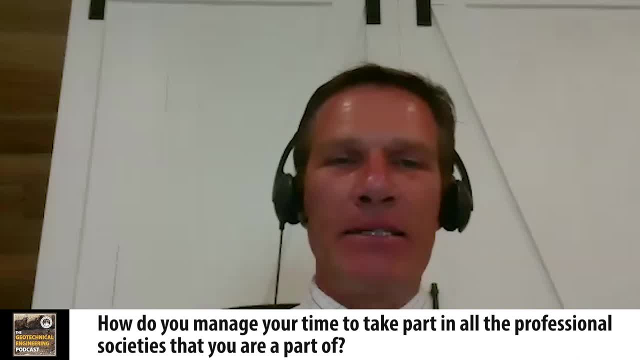 time to impact practice or impact society, And so that's. you mentioned us getting involved in the organizing committee for the 2019 Geo Congress. You know I thought by being on that committee we could bring in some fresh ideas, and you know we spend hours talking. 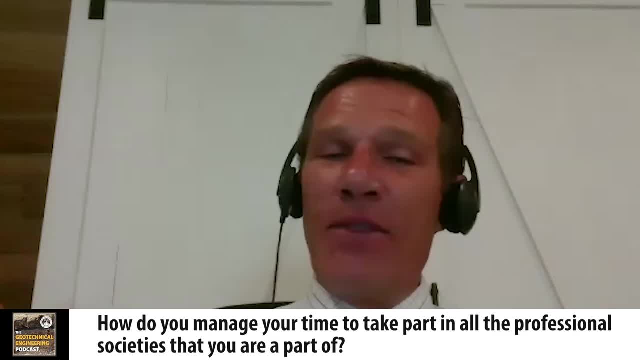 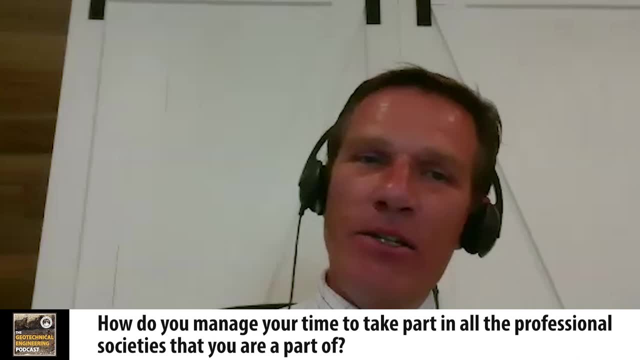 through how to best do that, Whether it's the geopets or the other things that we spend hours talking about. you know it's a lot, it's a good amount of time to spend, but we- I think we- changed the way that. 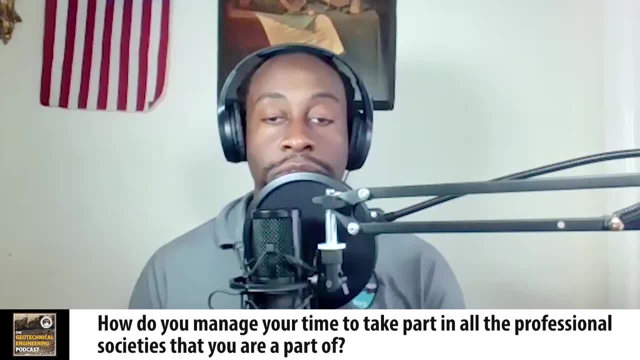 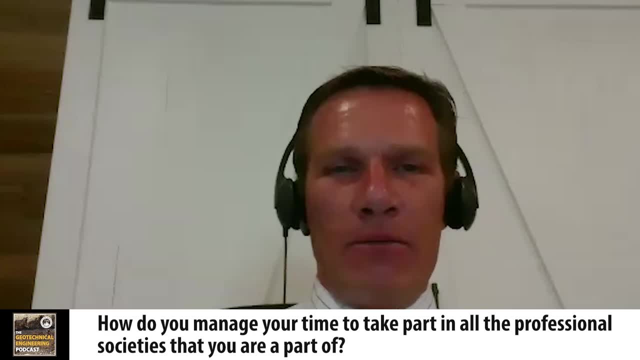 the ASC is going to do things in the future And- and I kind of look at it that way- that that you know, there's, of course, the importance of networking for a lot of professionals and that's why they spend their time on that. For, for me, I look at it as, yes, I need to network. 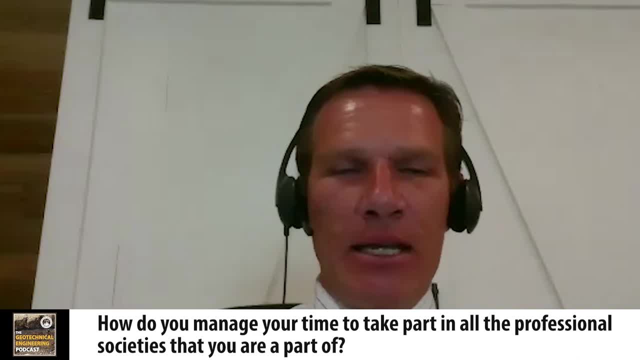 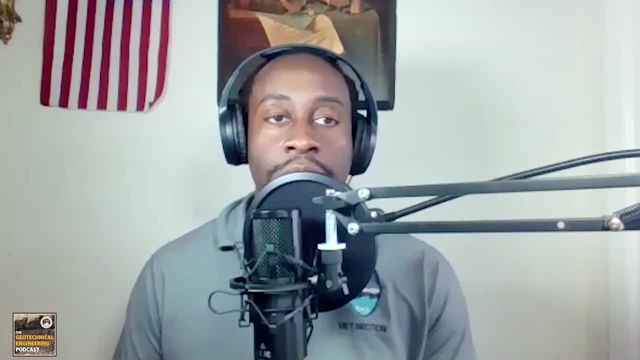 but also I want to try to make some kind of impact, So I get involved in things where I can hopefully make a bit of impact. It's powerful. That's powerful. I think that you know, especially some of the younger listeners. 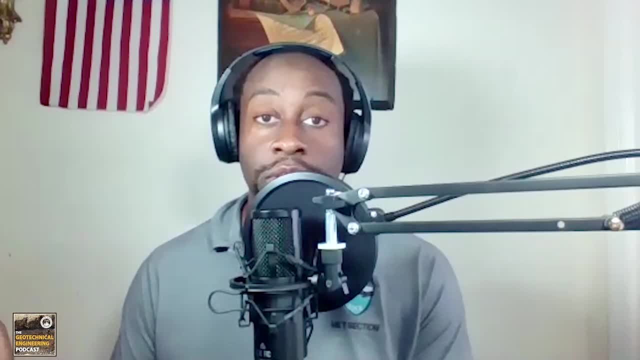 you know they, they realize that. you know I have to go to the field, I have to learn my craft and then I have to, you know, find times to do other things. And I think that what you're saying makes a lot of sense. It's like if you're passionate about what it is you're 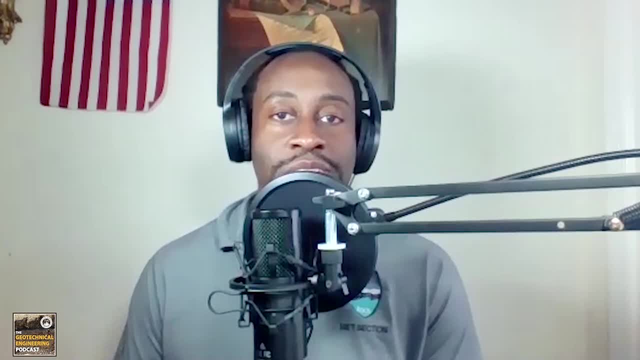 doing, then it makes it a little easier to spend the time doing it. But if you're not checked into what it is you're trying to do, then it's a little easier to spend the time doing it. It's just it's going to feel more like a chore than something you enjoy doing. 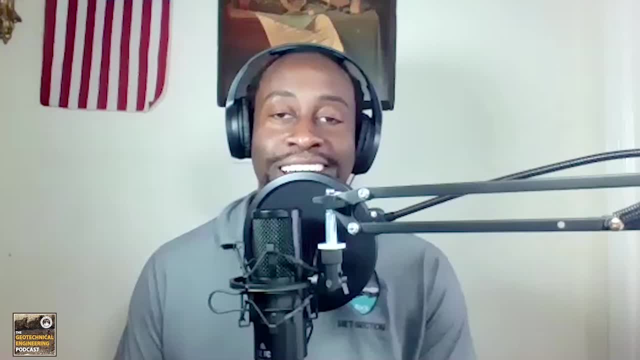 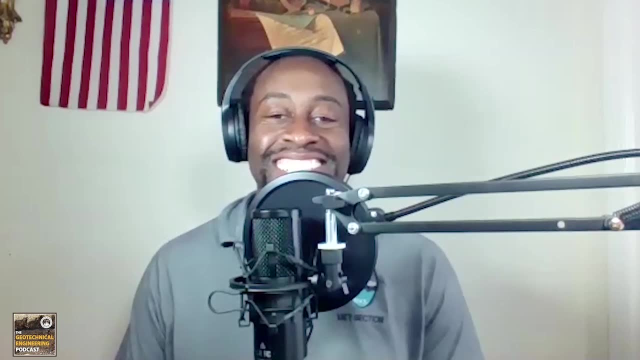 And I think we've all been there, And those are the kinds of things you just put off and then you just make trouble for yourself and others. So I've tried to narrow it down just to things that, like you said, are are that you're passionate about, And for me it's that. 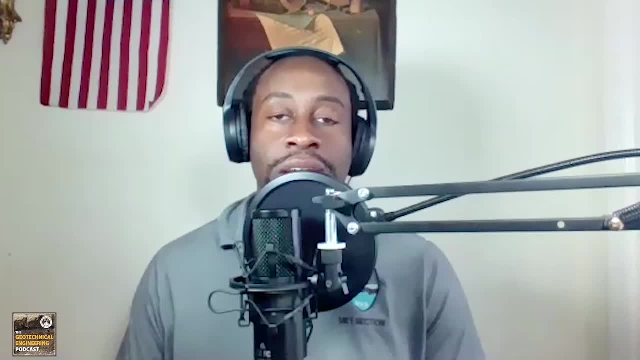 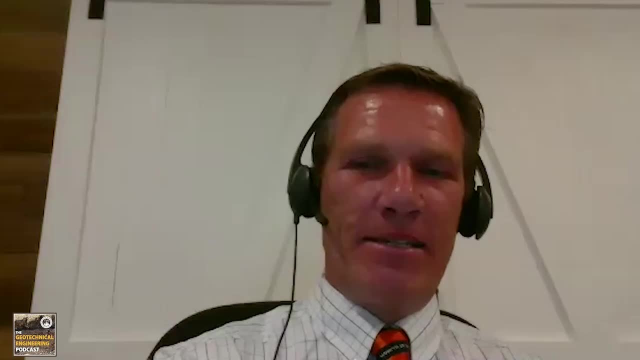 I hopefully can make a bit of an impact. Excellent, Excellent. We look back at your career. Is there anything you can think of that you wish you knew then, that you know now? Wow, that's, that's always a tough question, You know again. I think it goes back to that. 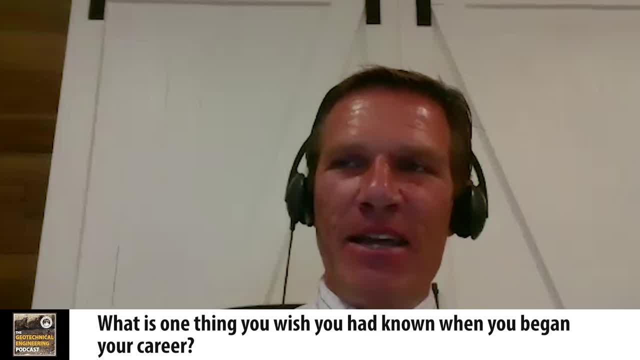 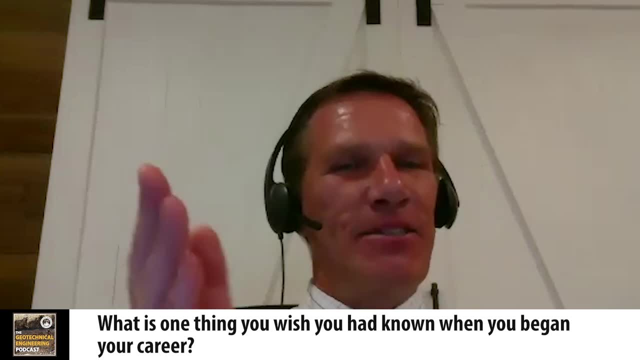 idea of change. that that well, I think maybe from an outside perspective, engineers are seen as kind of static and stoic at the same time and not big fans of change, And I think I would count myself somewhat in that category. But understanding that, even as an engineer, that the profession 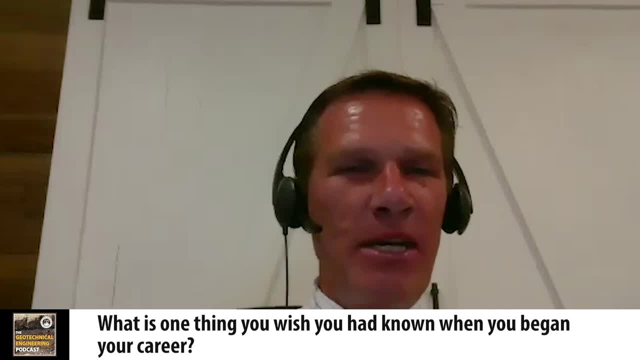 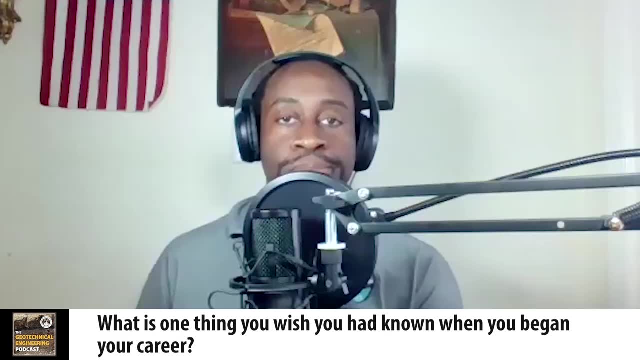 is constantly changing. You need to change to keep up with it. You need to expect that. whether you're in practice or research and academics, I'm constantly learning new stuff. I'm involved with a project now where we have or we're going after a project where there are. 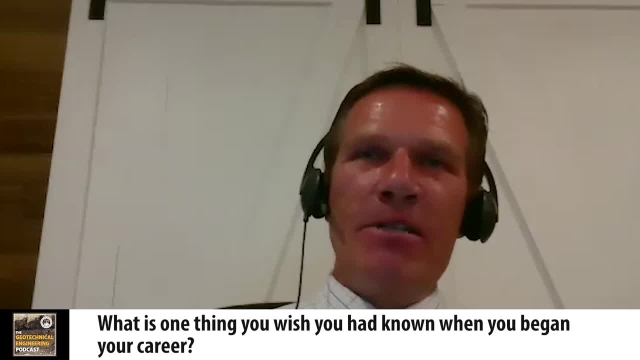 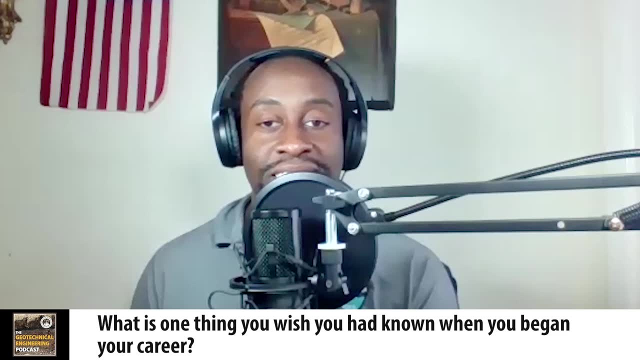 colloidal scientists, chemists, physicists and geotechnical engineers involved and trying to tie all these things together, And it's really kind of so. I've had to learn about colloidal science. I've had to learn about nanoparticles. 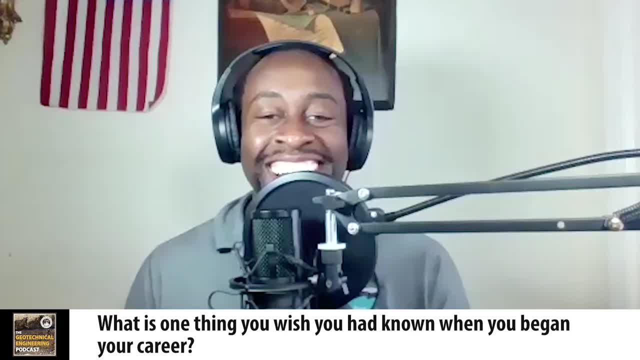 I never thought I'd ever touch, But it's, it's an interesting opportunity And I said: well, you know, this is research, So you know, why not try learning something new? And it I I came to. 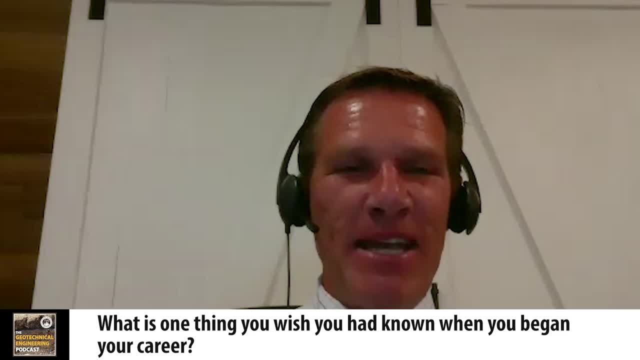 realize, especially as we started talking about this opportunity to do this podcast, that that is the constant It's. it's that you're always learning And- and I wish I'd have known that earlier, Some of the learning might've been less painful. 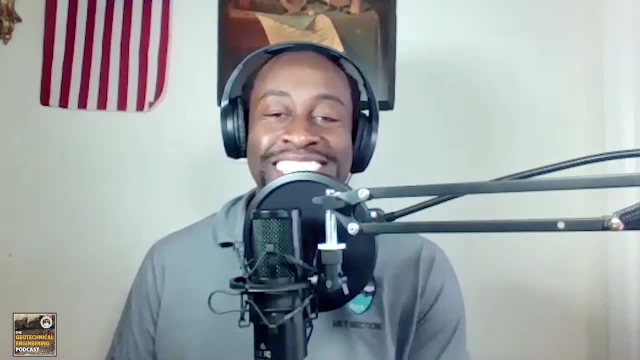 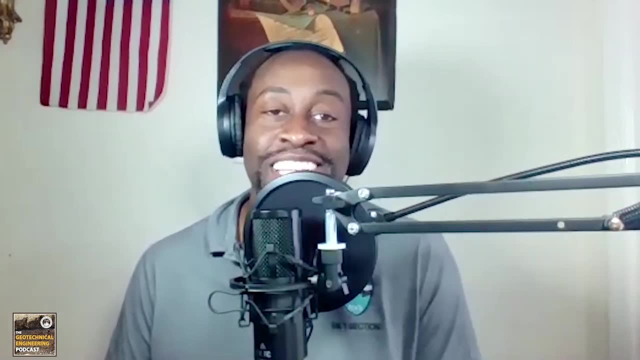 There you go, You have a PhD, professional license engineer and you're saying: you're always learning. You never get to that point where you say, all right, turn off the learning meter. It's like we're going to keep taking things in And that's great. I think that's. 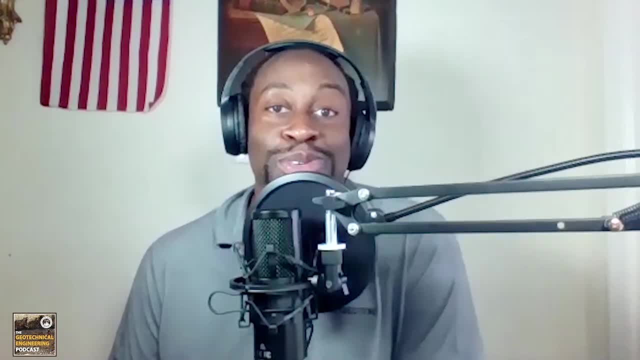 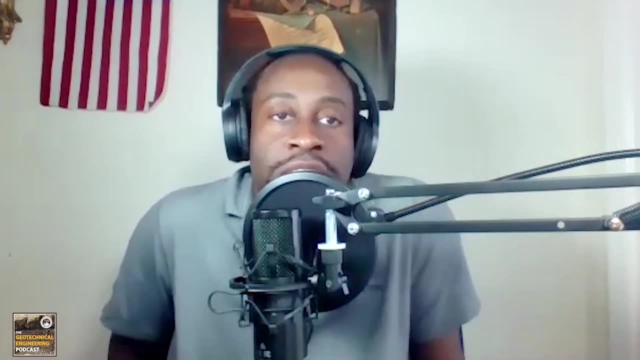 what really keeps us all sharp and checked in, because you never know what you're going to be doing the next day. So that's pretty cool. That's pretty cool. What advice would you give to a young geotech comes into your office and says you know, I'm at a point in my career? 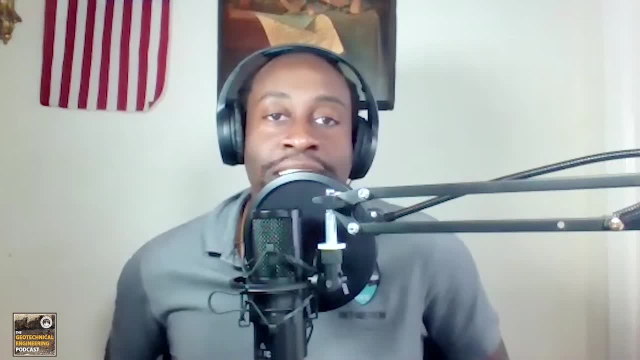 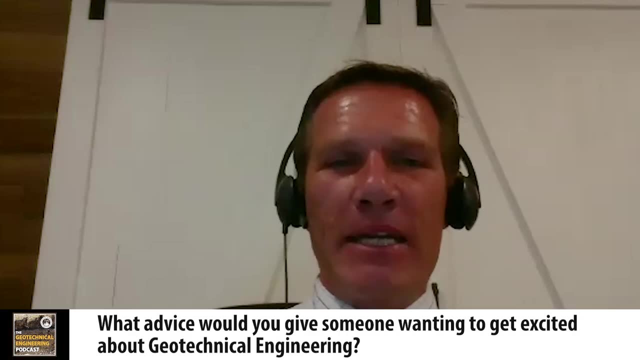 where you know I'm trying to get excited about geotechnical engineering. How do I get excited? What are some of the things you would share from an advice standpoint? Well, the the first thing I share is is my story, because I think it's not that unusual. 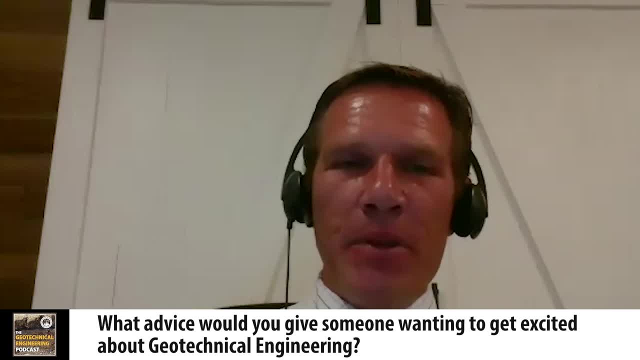 So when, when I started in civil I I like most everybody else, you think civil engineering, you think structures and you think environment- I started on the structure side and I got into some of those structures, classes and the instructors say, well, open up your code book to. 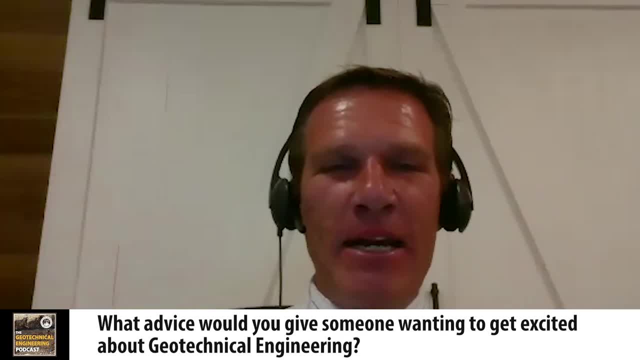 to section a, point four, point three, point B, you know so on, And I was like: is this what civil engineering is really about? And even for structural engineers, obviously it's not about that. But when you start the education process with a code book, I was like that, that really. 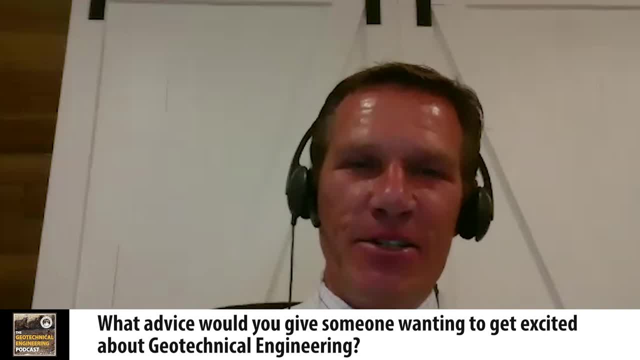 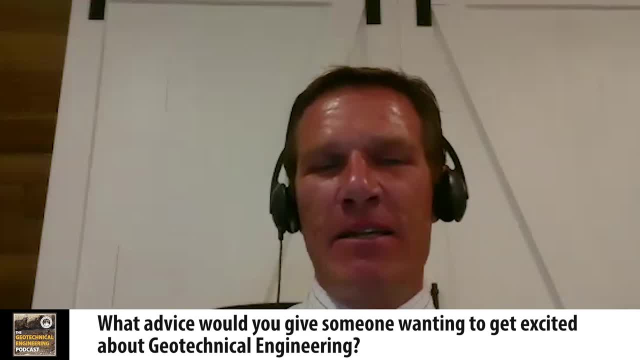 artificial materials that we can specify such that you know only 5% variance from your ideal parameters are accepted on a project or it's got to be better than that. You can only have like a 5% failure of you know too low strength concrete steel that doesn't meet your specs We don't get. 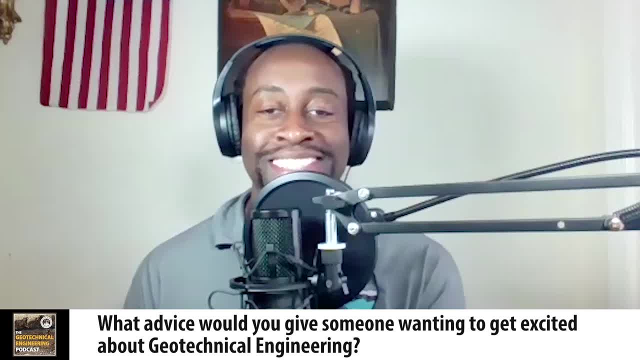 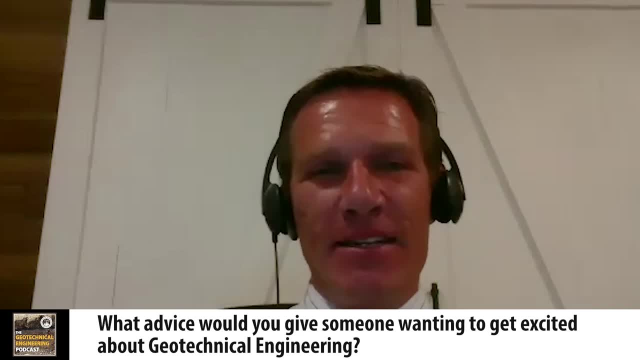 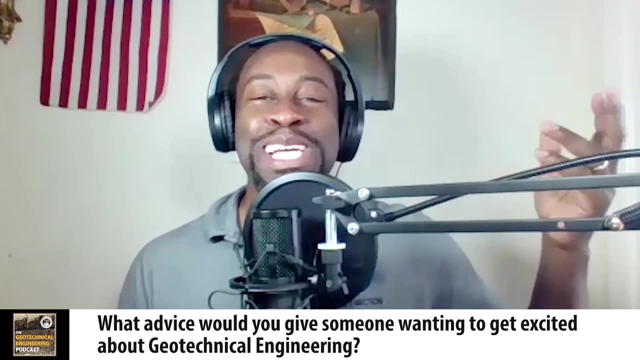 that in geotechnical engineering, Not even close there, Yeah, exactly, Not even close. Yeah, And that that uncertainty or that that variability really attracted me. Uh, and the fact that there were no code books. Yeah, It was like, you know, pass me the, pass me the geo codes. Like, yeah, we don't have one of 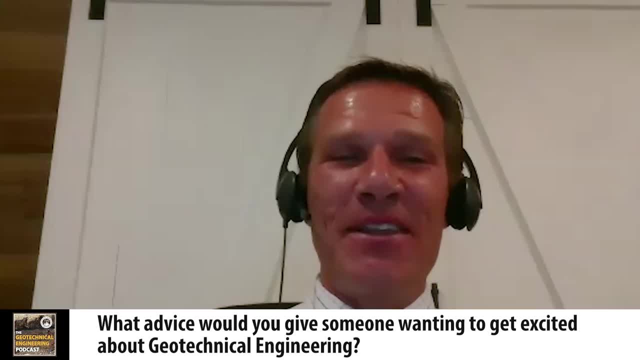 those. Of course that we're working on those sorts of things, but the the way I look at it, the purpose of developing those codes is to make sure that engineers recognize that uncertainty is throughout our profession And we're trying to find, we're finally trying to quantify. 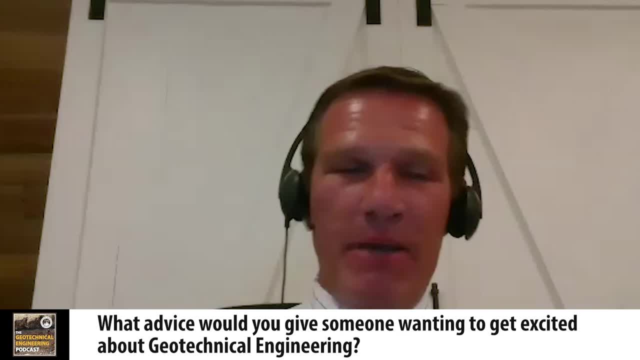 that uncertainty instead of just Using big factors of safety or saying it's all engineering judgment. Yeah, And I certainly do not want to ever cast aspersions on engineering judgment- I I think it's critically important for engineers to have engineering judgment, particularly geotechnical engineers, because 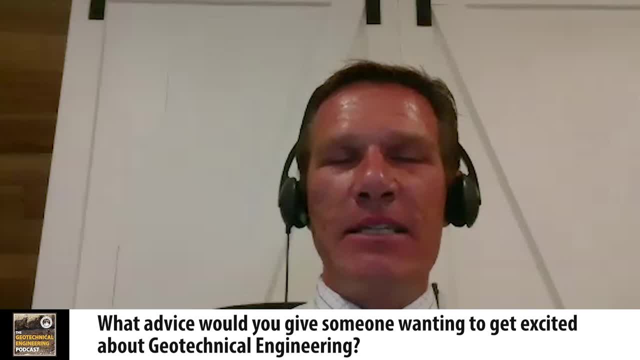 every site, every, as I tell my students- you may sample 1%- probably much less than 1%- of a given project site that you're going to influence With some structure. out of that, you may test 1% of what you've actually sampled. So if you're 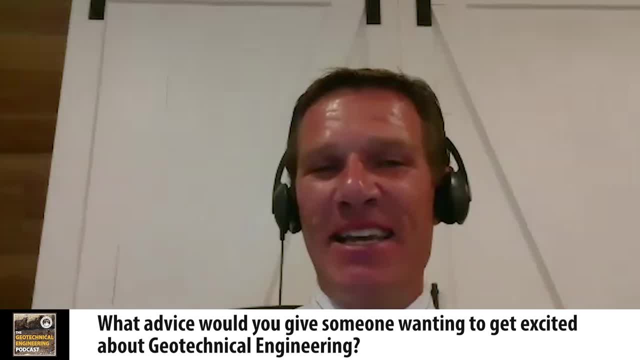 drilling 10 borings across the site. let's say that's 1%. Okay, Probably only going to test 1% of what you've actually drilled, because you're taking samples every five feet or whatever it is, And you're saying you're testing only a fraction of those samples you retrieve. 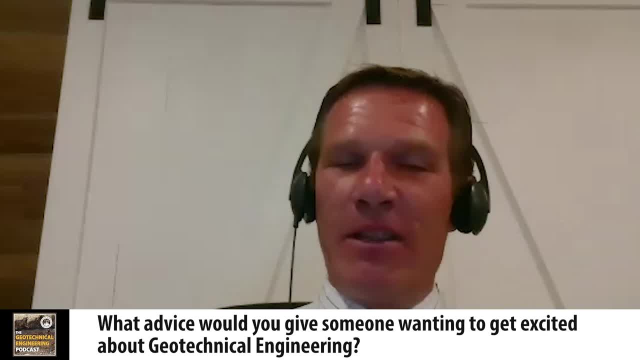 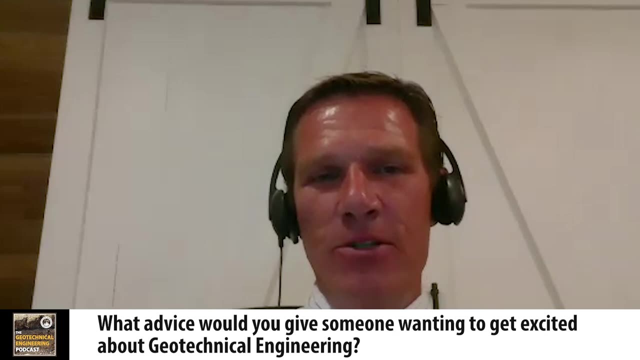 So it really requires a thorough understanding of a lot of different areas, from geology to understanding soil Mechanics, rock mechanics, structural engineering, hydro systems engineering, all of those kind of roll together- to become a good geotechnical engineer And so that that variety and that 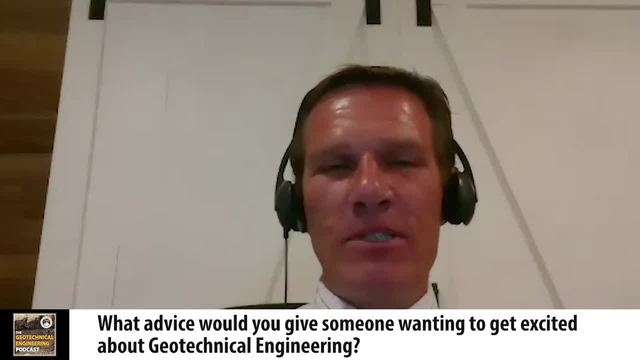 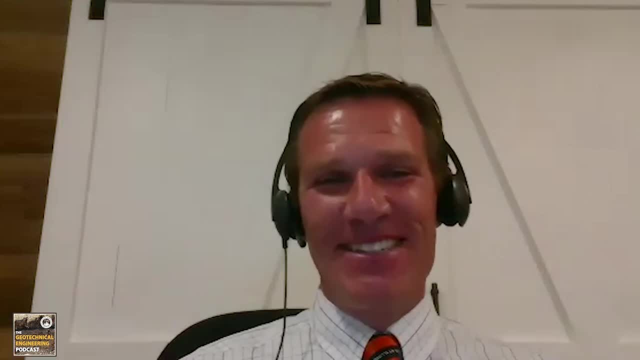 that uncertainty really attracted me, And if those things don't scare a student off or somebody who came into my office asking about it, that doesn't scare you off, Maybe this is the right field for you. There you go. It's either going to scare you off or excite you, So that's a good way to put it. 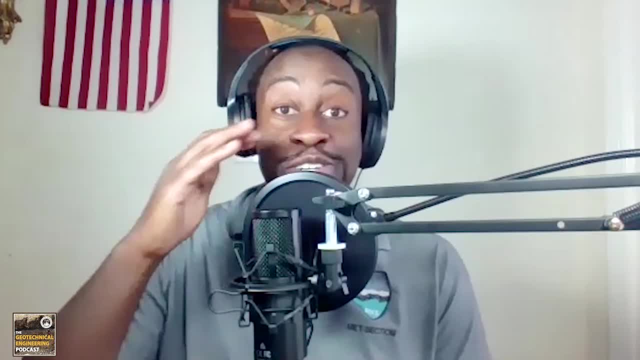 It's a good way to put it. Yeah, You think about it is really not a lot that you're using for this design. So there's a lot, of, a lot of other variables that come into play. Right? That's great. 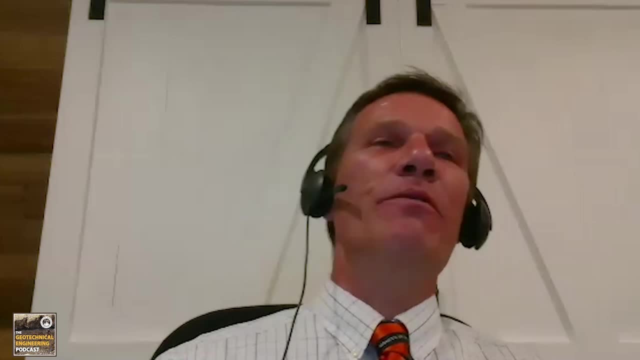 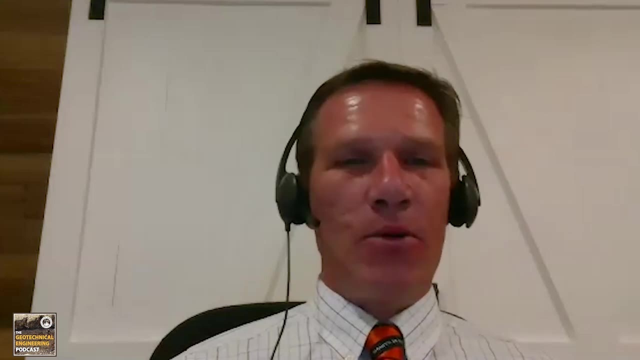 And you know when, when students ask me about all the new development. well, some will ask me about new developments in geotechnical engineering, like biogeotechnics or geosynthetics a few years back and other things that are new. I keep coming back to the same same answer: that if you understand the fundamentals of 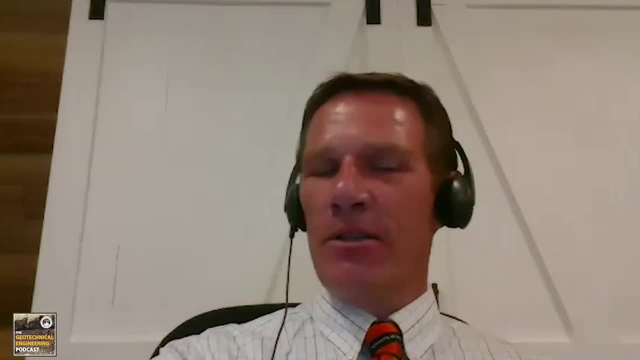 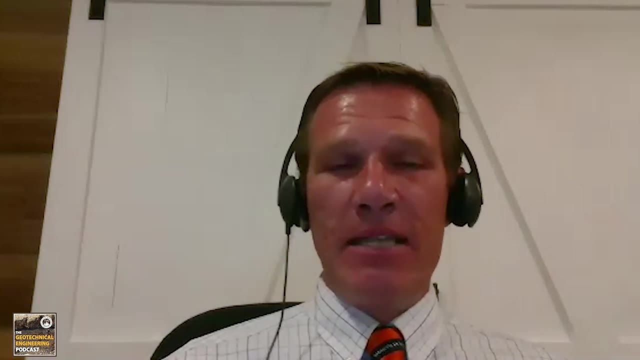 these: the soil mechanics, rock mechanics, geology and those others that I listed. if you understand those fundamentals, you can then learn all these other new things that come up. that is not that difficult if you have a good grasp of how soils behave. 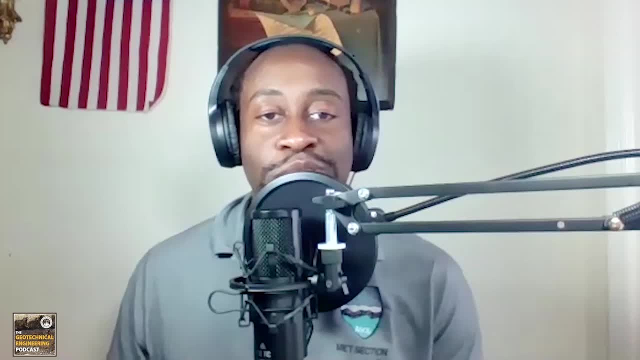 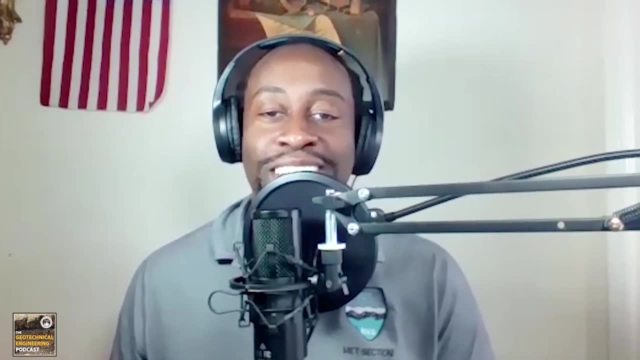 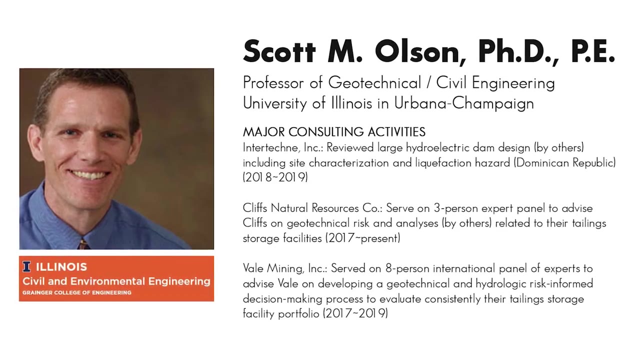 Well said, well said Well. thank you so much. We're going to come back in just a minute to close this one out with Professor Olson and our career factor safety end segment. Stick around, Welcome back. It's time for our career factor of safety end segment. 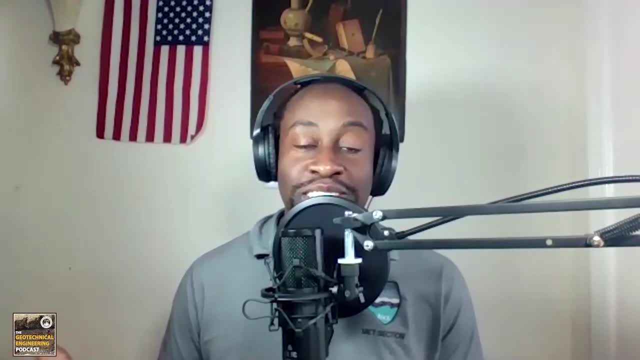 And in geotechnical engineering, just like many disciplines of engineering- we hinted at this earlier- it's important to incorporate a factor of safety into your design, But what about incorporating a factor of safety into your career? So today we're speaking with none other than Dr Scott Olson, PE. 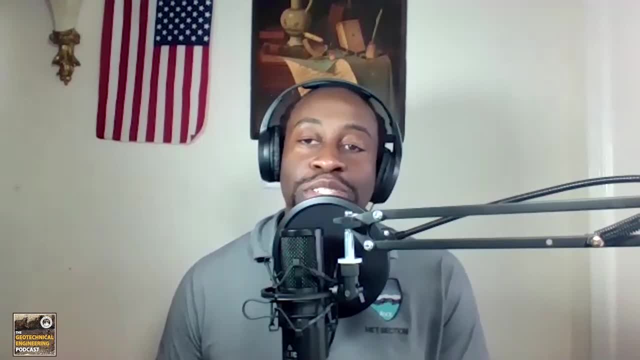 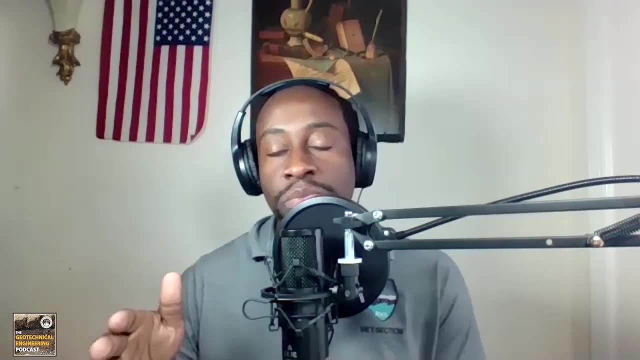 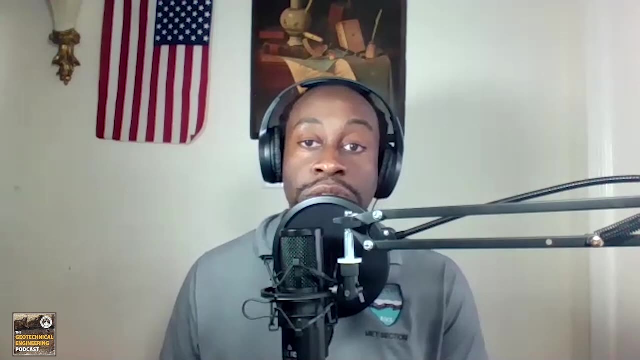 Professor, we spoke to you earlier about the things that you accomplish in your career. What advice would you give to people who are interested in engineering? What advice would you give to geotechs, listening for how they can advance their career, And that could be moving up in the professional world or moving up as a professor, or maybe even making a change from, you know, professional to academic, as you did? 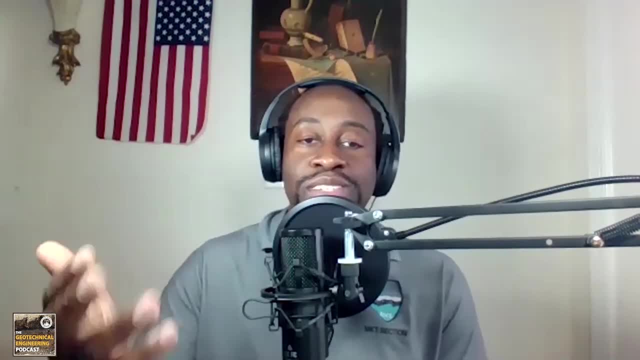 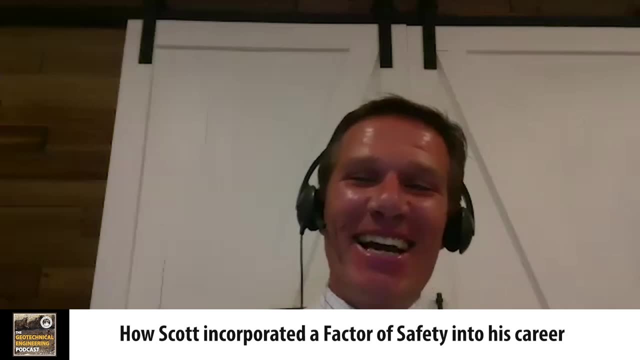 And how can they do that to secure a factor of safety in their career? That's an interesting way of putting that question. I had not heard it that way before, but I like it. I'm going to use that, if you don't mind. 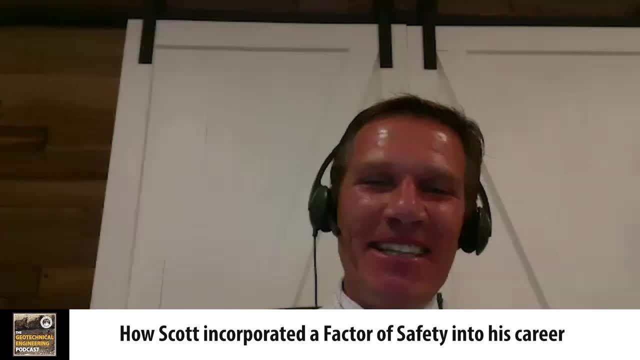 Go ahead, go ahead. The two things that I like, The two things that I always encourage students to do when I put on that mentoring hat, is to first get as broad of an experience as you can when you go into practice. And so even my PhD students who really strongly want to get that first academic job and jumpstart their career academically, I push them as hard, as strongly as I can, without being too forceful- into practice first. 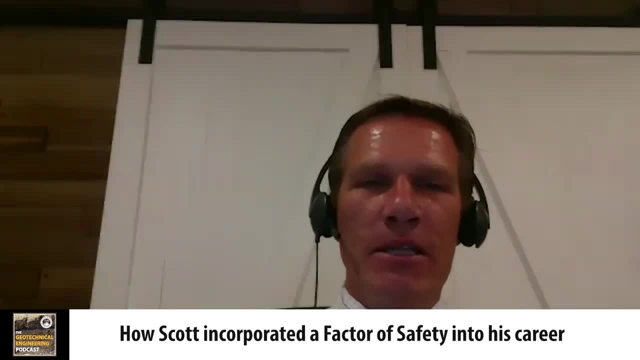 Because if they get into practice, even for just a couple of years, the experience they're going to gain And the variety of things they're going to see far outweigh what they're going to do those first couple of years in academics. And I always come back to one thing for those sorts of students is you need to understand what the questions are that you want to address through research. 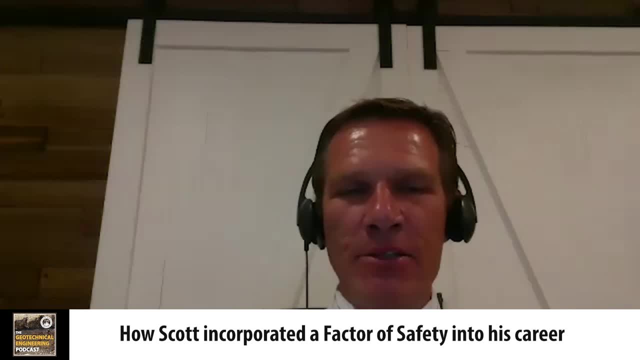 Where are the knowledge gaps? And if you don't understand where the knowledge gaps are, like I said earlier, the questions that you can't answer, And you get involved in a project and you just don't know what that right answer is, That's research. 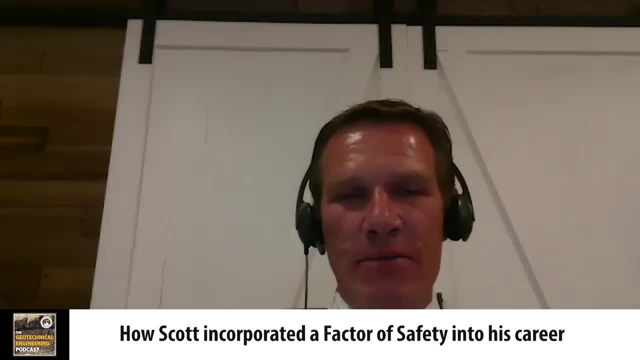 That then can develop into research. So a lot of my research has developed from those things that I ran into in practice like that. So that's one of them is that desire to keep trying new things, Because it just it will help you develop that engineering judgment that you need to have in this profession. 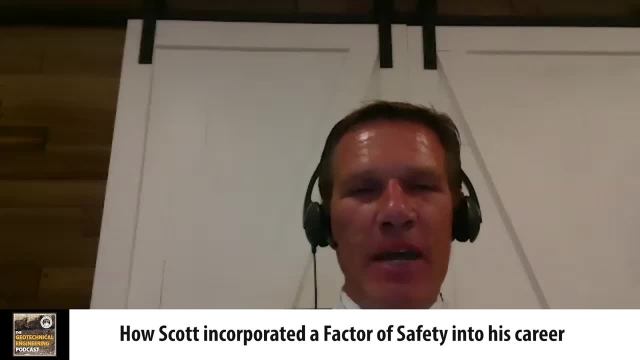 And then making switches. I've never been a humanist. I'm not a huge fan of making switches, And for me- maybe I've been lucky that way- That it's just keeping your eye open to what doors and what opportunities come before you. 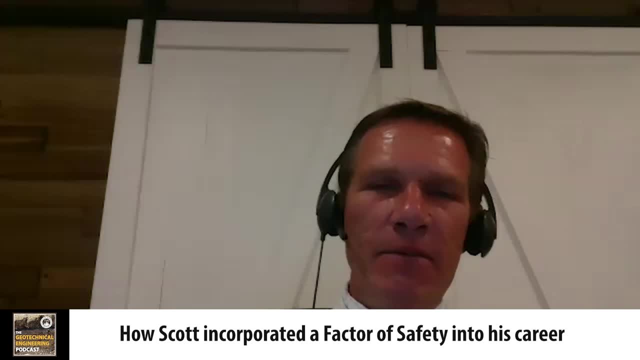 Because I strongly believe that even people that feel they're stuck, there's always an opportunity out there, Even if you don't know what that opportunity is. But if you prepare yourself to look for those opportunities and you're willing to walk through that door when it does finally open. 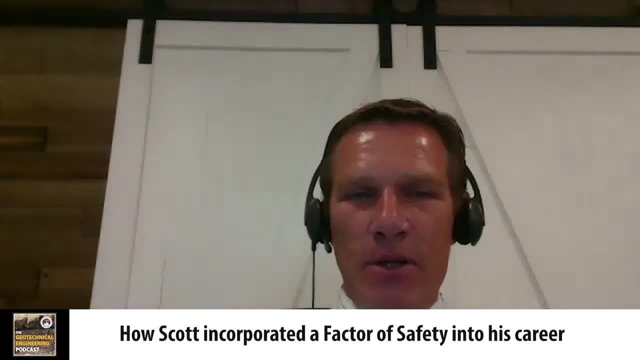 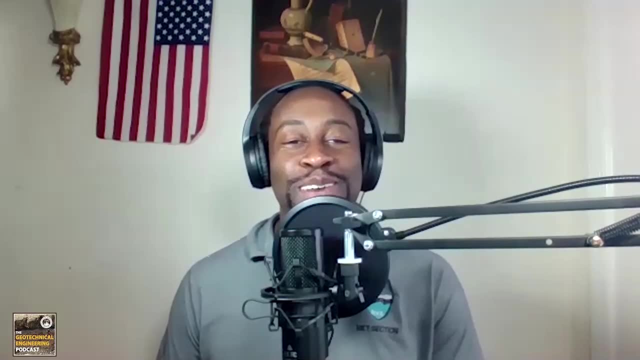 Yeah, Then you can make the change to make your- you know, to advance your career and add that factor of safety to what you're doing. Awesome, Awesome. Well, thank you so much, Professor, for coming on and sharing these great insights with us. 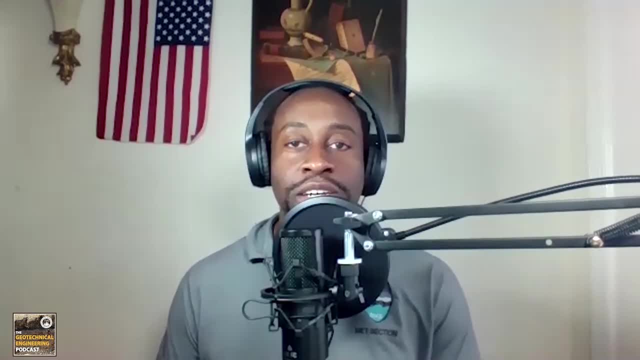 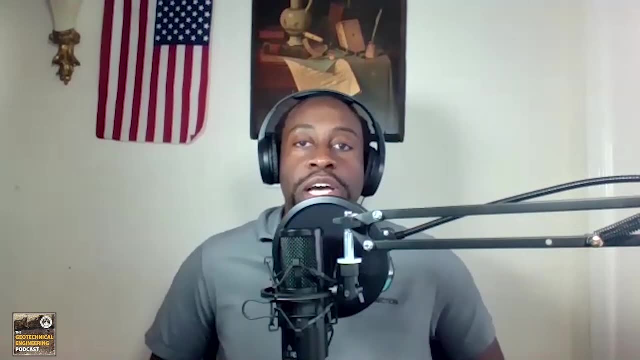 And thank you for all that you do as an engineer and impacting our great society. We appreciate that You've given some great information and great advice to our listeners. What's the best way for them to reach out to you if they wanted to learn more?